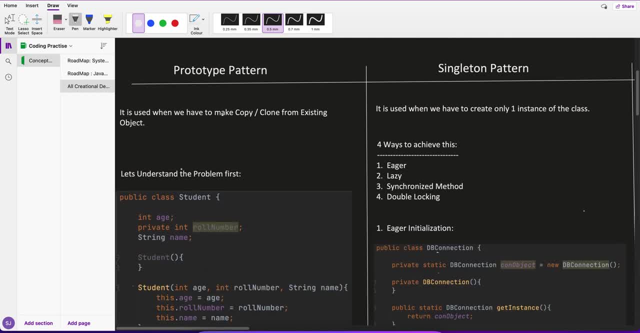 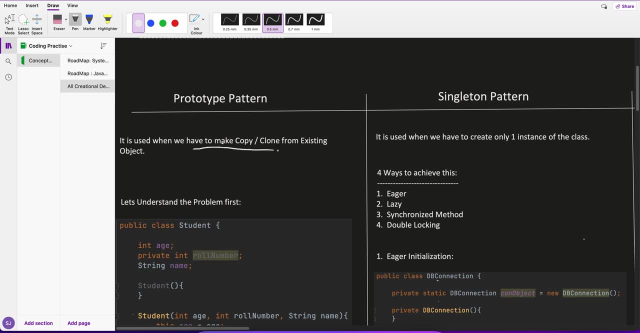 all the 23 design patterns, Most simplest, Let's check it out. So why it is used? So it is used when we have to make a copy clone from the existing object. Now consider that existing original object is your robot. Okay, and this is very, very. 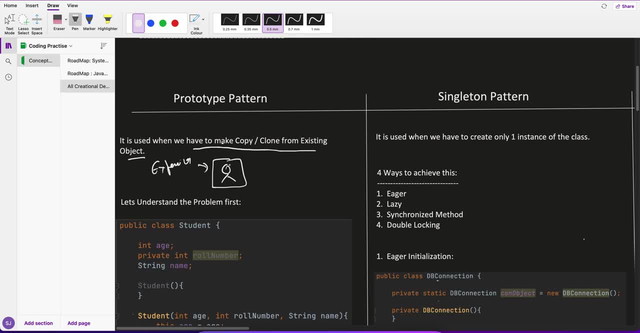 expensive object, very, very expensive object, to create a robot. But now you wanted to clone this and do some minor modification. So you, you should avoid creating new classes, right, just for the minor modification, Right? So what is the best way is that we, whatever the original, clone I have, whatever the original. 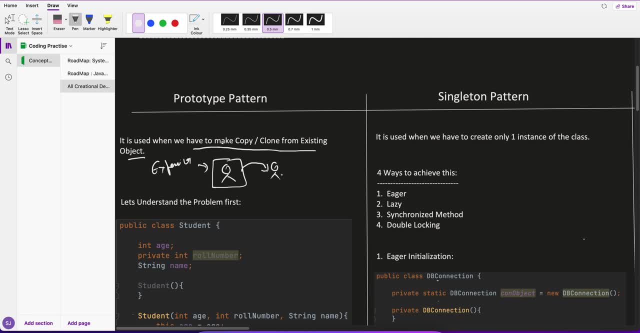 objects I have created. let's make a clone out of it and do certain minor modification. So if I want 100 different type of road robots on, so let's say this is my base Once I created the base- and this is creating a base is very expensive- Let's say I have created a base, Now I can clone it and do some. 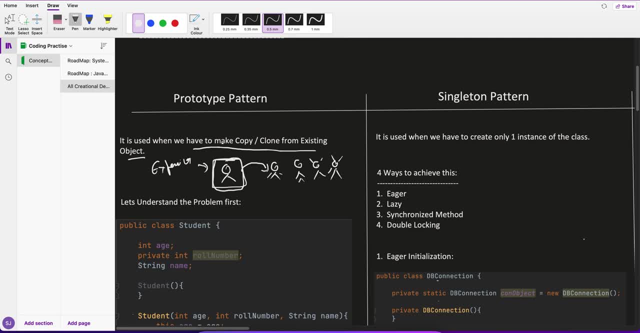 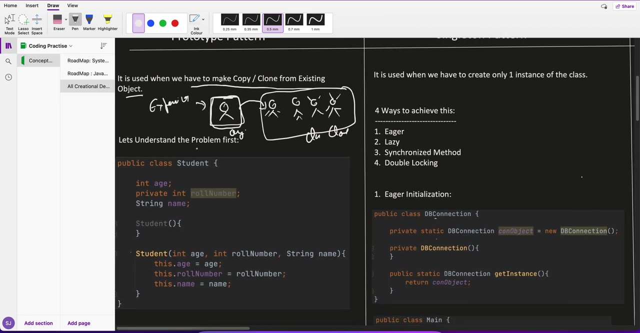 certain minor modification, that Okay, certain certain changes in different, different robots. Right, So these are the clone, These are clone and this is original. Okay, So prototype pattern is: it is used when we, when you have to make a clone from the existing object and creation of an existing object is very, very expensive. Okay, Let's first 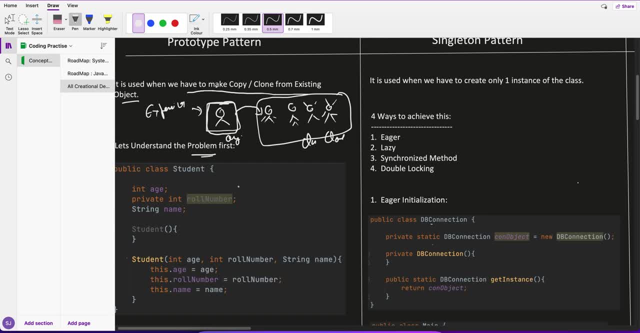 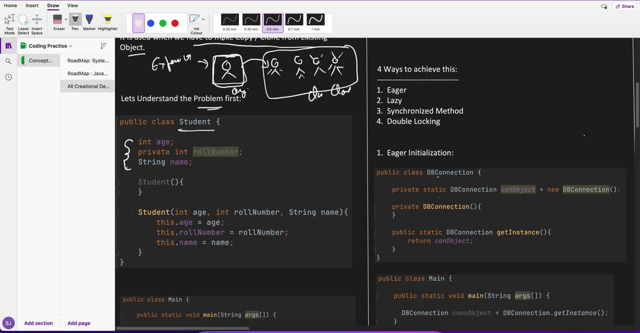 understand the problem and then we will see a solution for it. So very simple thing. I have created one student class. Okay, Let's say, student has certain instance parameter I have already created. So let's say, this is. I've created only three instance. 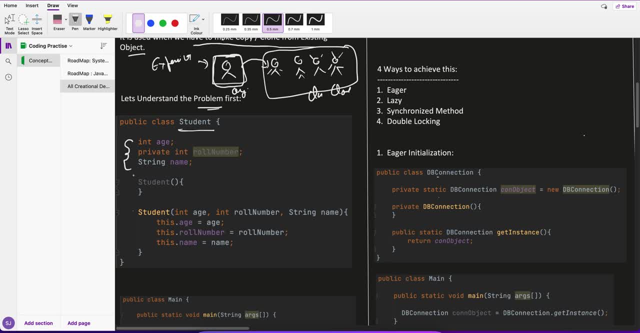 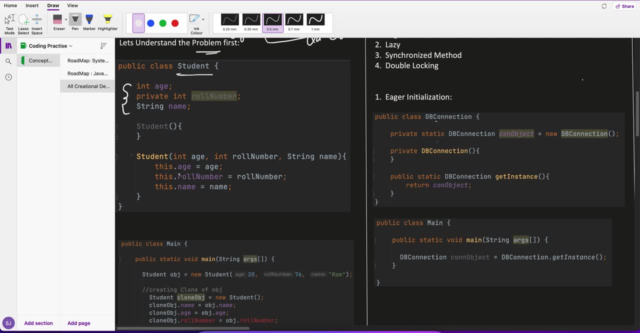 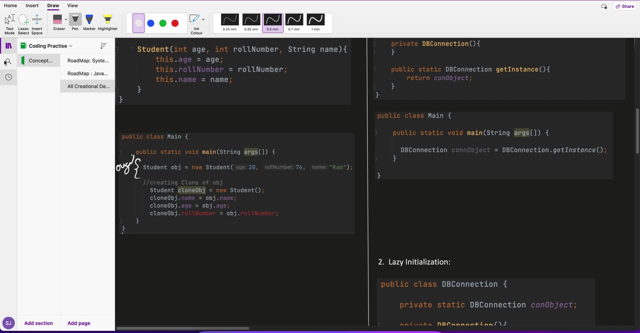 variable. But let's say this student object is very, very heavy and lot of instance variables are present, So this is one constructor which is used to initialize this instance variable. So let's say I am creating first original, So this is my original object. Okay, So while I'm creating an original objects, it's 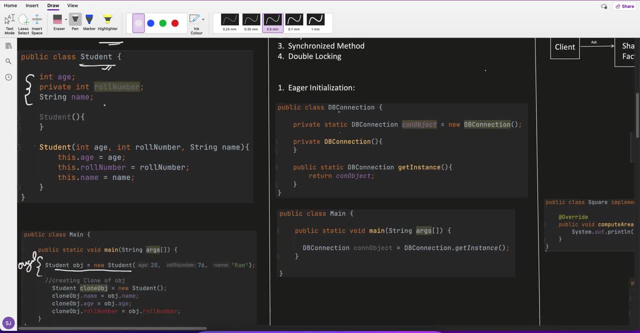 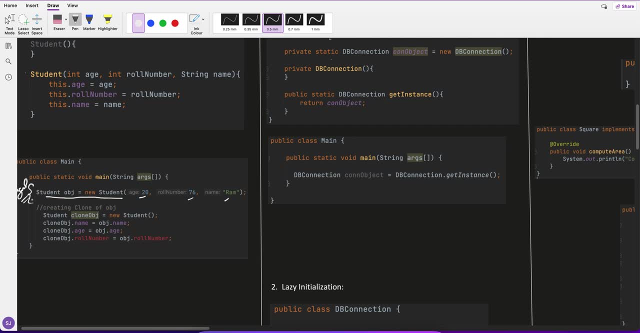 very easy. I'm creating a new student and pass my age roll number and name. age roll number and name. Okay, my original student is created. Now for original, I need to clone it. How can I clone it now? So generally, what we can think is, let's say I'm 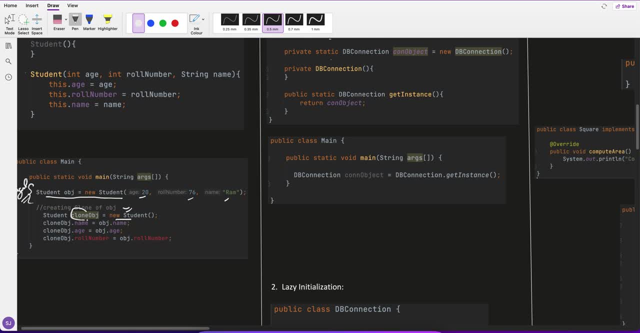 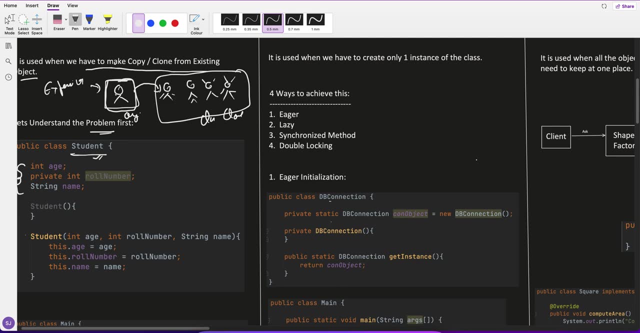 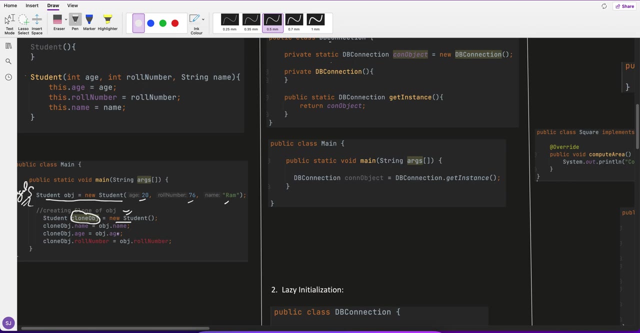 creating a new object, the student, which I give it a name, a clone, And its values, which I have to set, because all the this object I have created, it has certain, Let's say, properties. I want to copy that properties, Okay, want to call those methods again to generate that property. let's say something I can directly use. 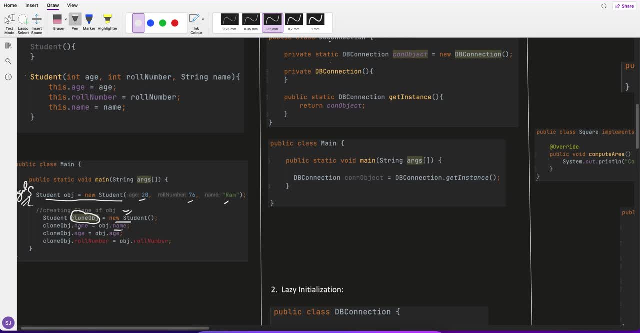 that property of the original and set into mine. so what I will do? whatever the clone objects I have created new a dot name from the original dot name. clone object- dot age- original dot age. clone dot roll number- original dot roll number. but here, if you see, one issue can come. I have 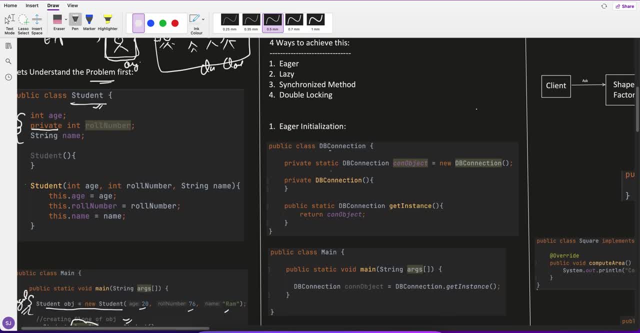 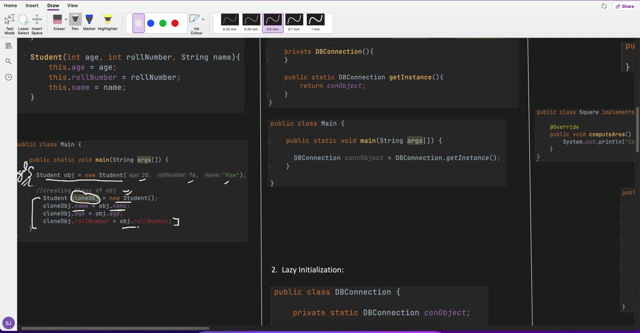 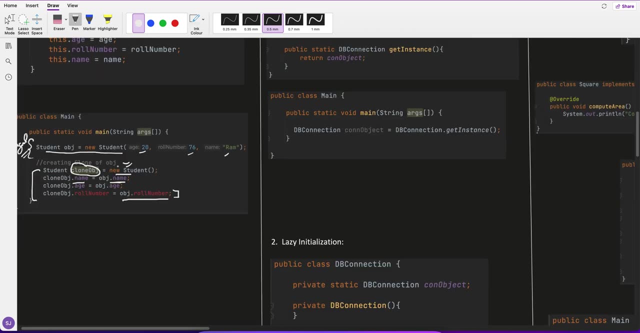 put the roll number as private. so one problem is like when you are trying to do a cloning by this, private members are only available within a class. outside this class you cannot access it. let's say, even if the getter method, let's say you can create that, okay. 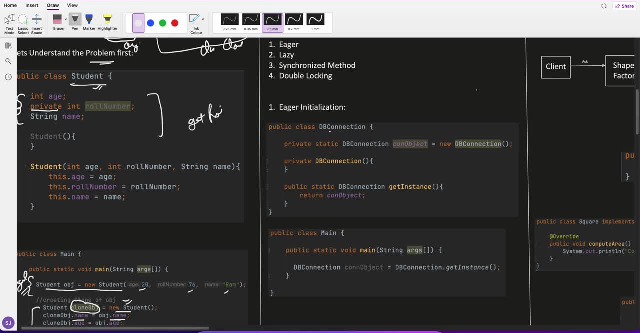 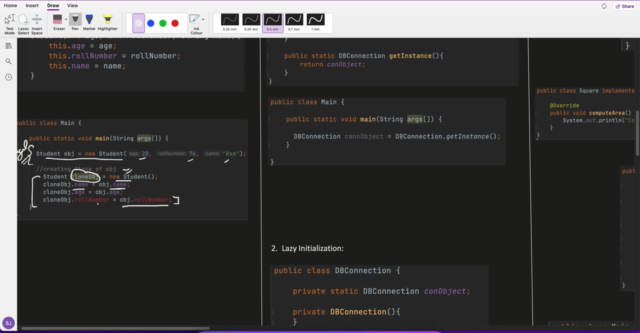 instance variable is private, but I can expose one get roll number method. but let's say that is also private. there is no way to access this, how you will copy that, okay. so this is one of the problem that in the current way of doing a cloning, okay, there could. 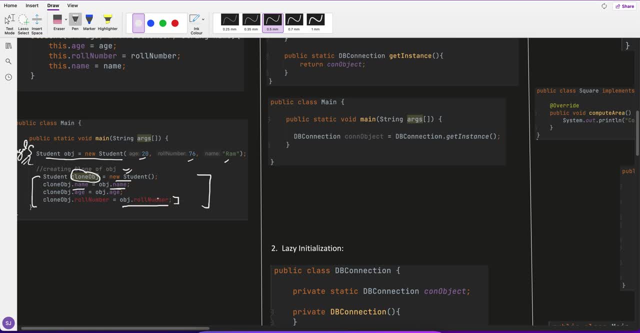 be a certain instance variable which is private and there is no way to access that, how you will set those values to your clone object. second problem you can easily identify from here is here the client which is actually doing the cloning. this has to know about all this original. 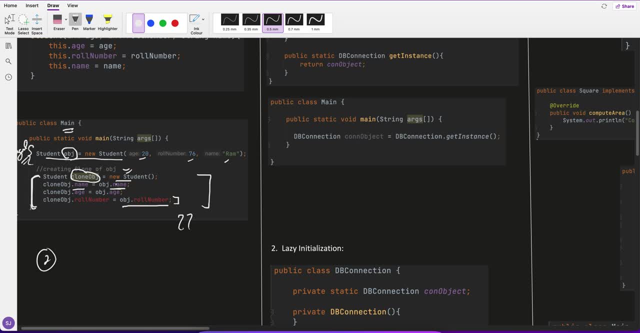 original object of it is creating. so in this there's a student. it has to know about all the student object. okay, it has name, it has age, it has role number, all the things which it has to copy like. what about certain logic? like this student class has 100 instance variables, let's say age. 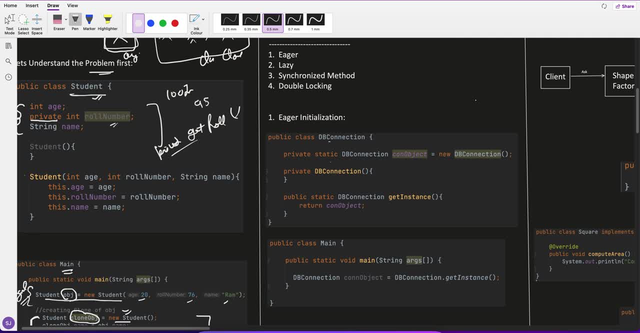 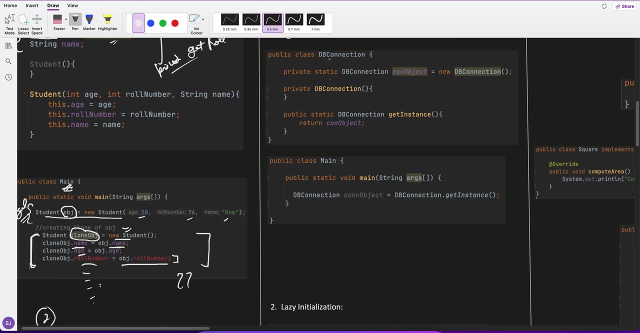 role, number, name, address, like this, and out of this, only 98 has to copy 2 doesn't matter, it doesn't have to be copy. so how this client has to know that, okay, only 98, i have to copy 2, i have to left. so means this client has to know about the exact student object, what all fields i have to copy, what. 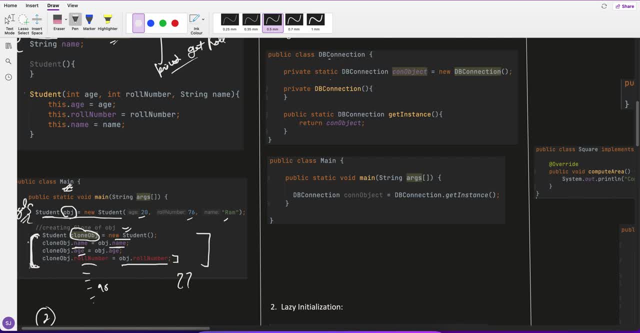 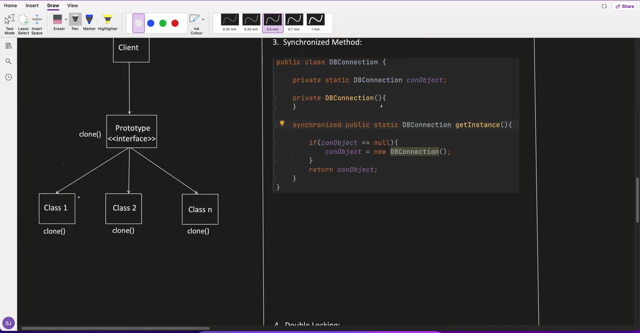 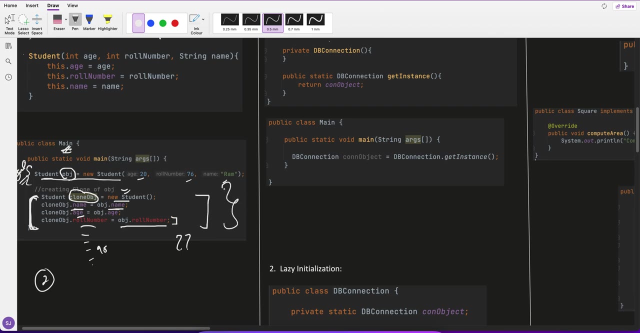 all fields, i have to leave. okay, so this is the two problems in the existing cloning. okay, now let's see how the prototype has resolved it. so, first of all, what prototype told? is this cloning logic? where i am doing right dot name equals to this. so this cloning logic should not be the 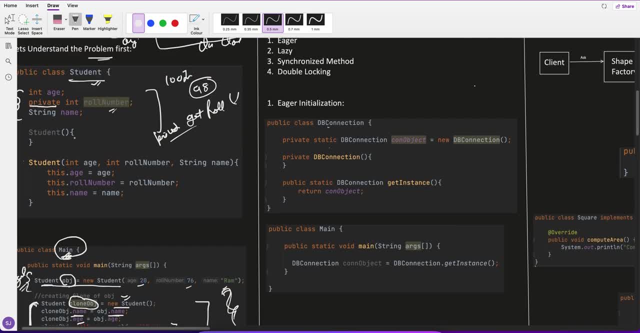 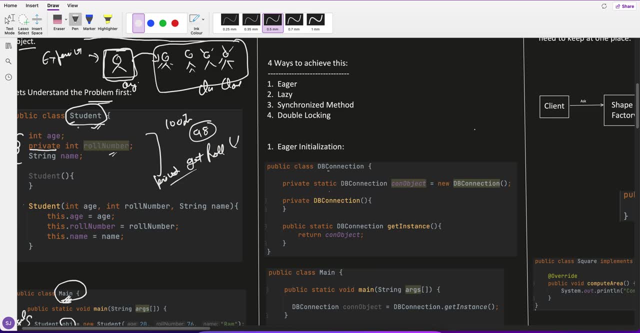 responsibility of the client. so this is: the client has to know about the exact student object. it should be the responsibility of the class itself, the original object which we are trying to clone. so in this case, so let's say this is our student class, let's say another class i want to. 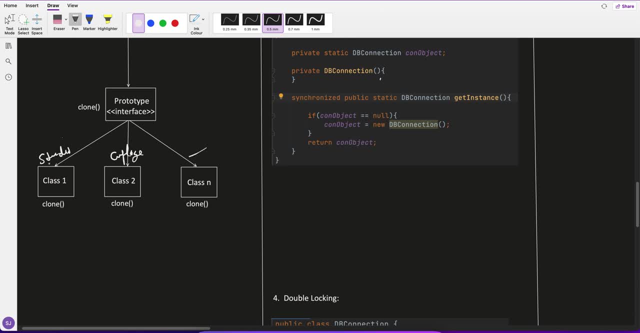 support this, let's say employee and some other class. so in all the original object class in which i have to support the clone, i have to expose one method, clone, and this has to actually do the clone. why? because first of all, let's say, in a student class, i am exposing the clone method. so all 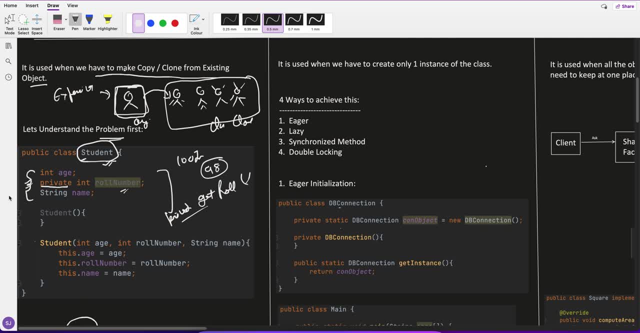 the private methods can also access it. that is one advantage. second thing is, since this is the same class we, it has also exposing the clone. it knows about itself very well, all the fields i need to do the cloning, all the fields i don't have to do the cloning. so all this cloning related logic. 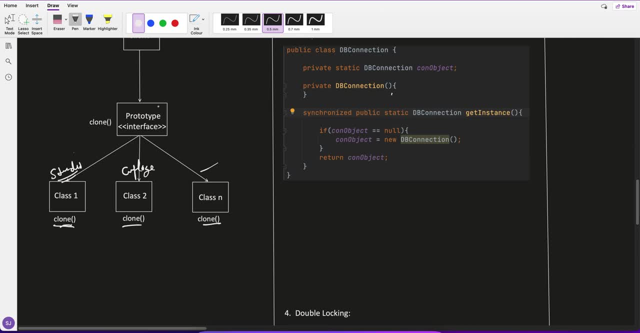 will be inside this, only okay. so why we have created one prototype interface is like: if this is not exist, then let's say student method will say: get clone. this will say that, okay, only clone. this will say that okay. let's say another class says that okay, do clone. 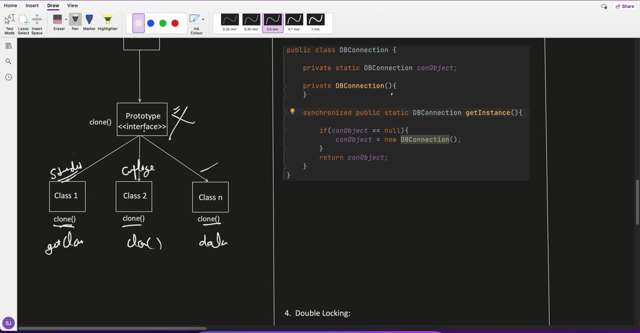 so there is no consistency. so let's say, with the prototype interface it says: says that one method, clone, and all are implementing it. so everybody has to implement clone. so there is certain consistency also comes into the picture. okay, so now for all the classes which you have to. 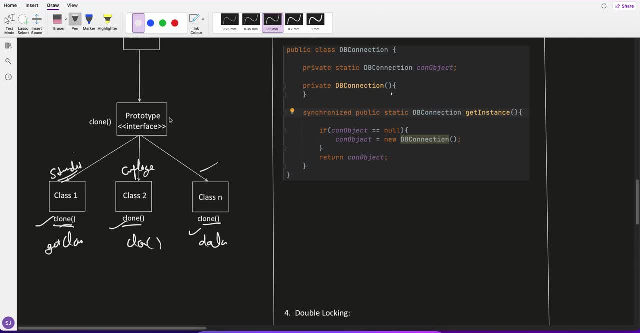 support the cloning. what you can do is you can create one prototype interface and expose the method clone and all the classes- in future also- which you want to support the cloning. you can implement that prototype and inside that you have to implement the cloning. okay, now the client will. 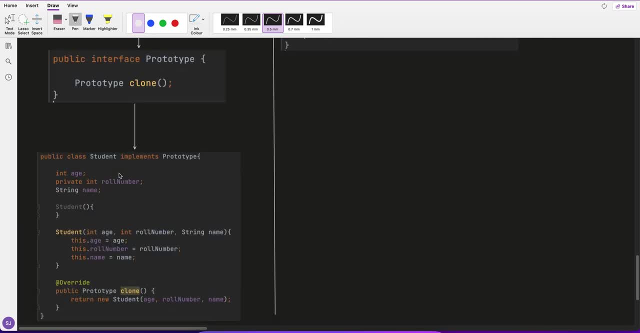 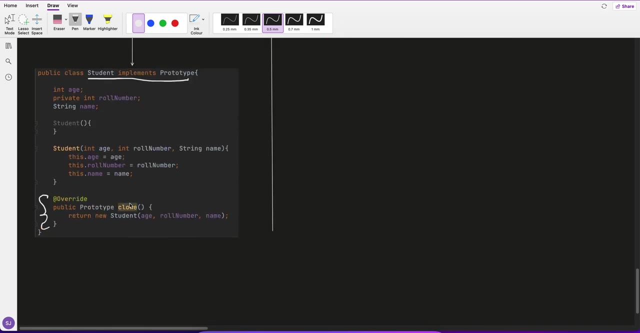 just simply say that clone. now let's see an example. let's say i have a method prototype and i have exposed method clone. now for a student i need to support the cloning. so student implements prototype, so i have to implement the clone method. so now let's say this in the main: first, 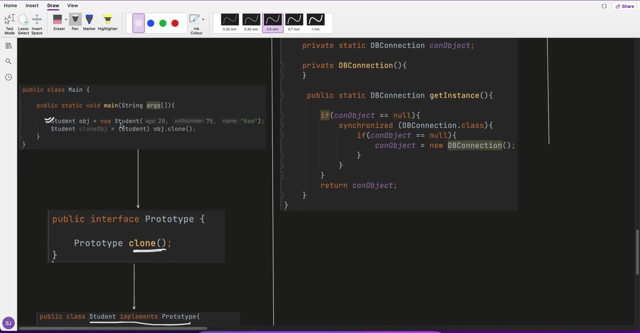 i created the original object: student, new student age, role, number and name. so my original object is created. now i want to do a cloning, so i want to clean a clone object. now- see how i am doing- is original object. so whatever the original object you have now, it is taking the responsibility of. 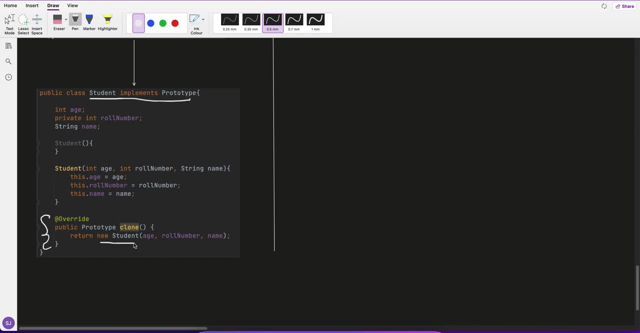 so this will call, and it is. it will create new student. hey, create a new new object- the student, but with all my properties- age, roll number, name. so it will set all these properties. so now here, if you see that now client doesn't have to worry about all the private parameters. 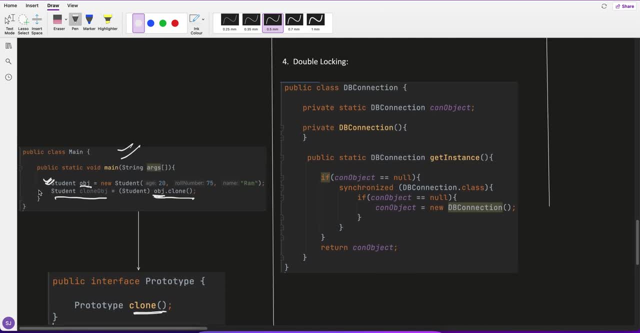 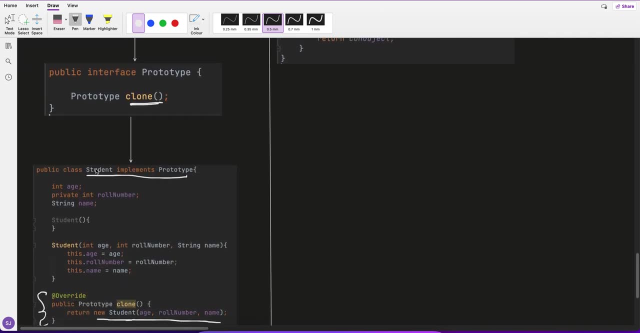 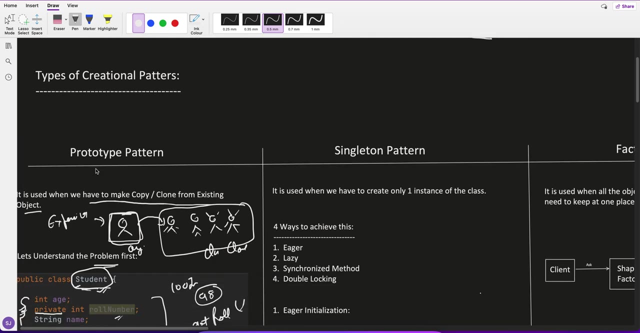 client doesn't have to worry about. to understand the student, what all fields I need to copy, what all fields I have to leave all this logic. this student class can take it okay, very, very simple. this is known as prototype design pattern. okay, now let's see what all the other design. 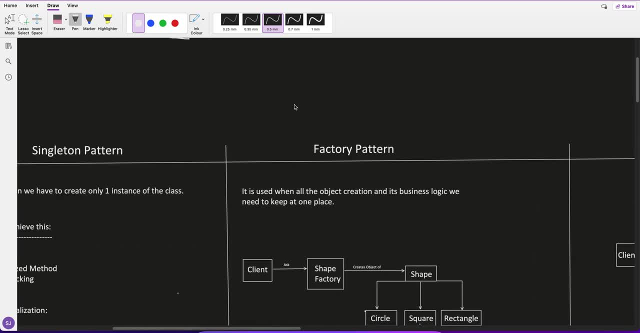 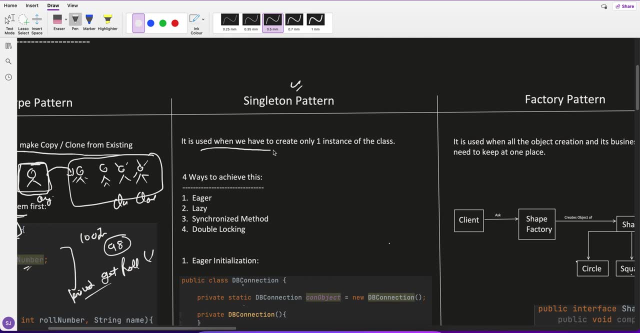 para uh, creation design patterns, which we have covered and let's see a quick overview of it. so now, what is the use of singleton pattern? singleton pattern, as you know, it is used when we have to create only one instance of the class, so there are many, many use cases. you 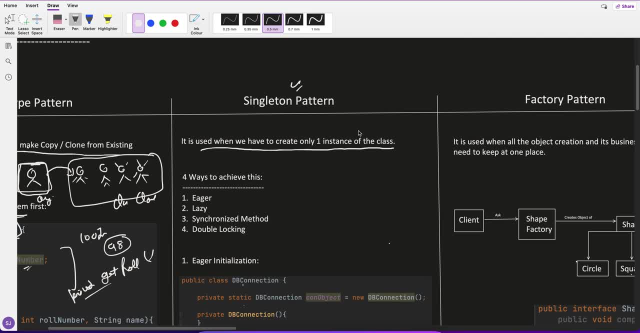 will find where you have to create only one object, right? let's say DB connection, you want only one DB connection, and then you can do, perform any operations. let's say ATM, so you want only one ATM. let's say another thing, you which, you want this. okay, so in that case, what you will have? 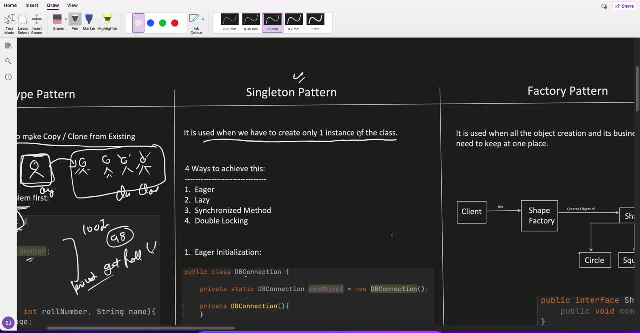 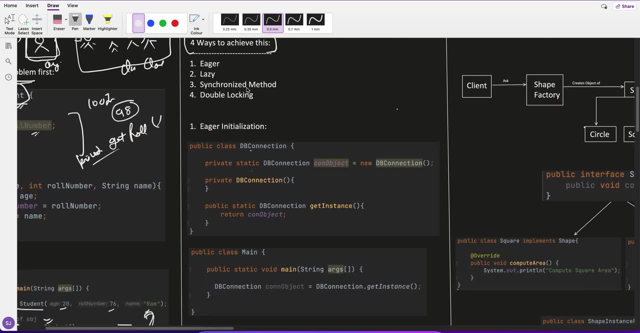 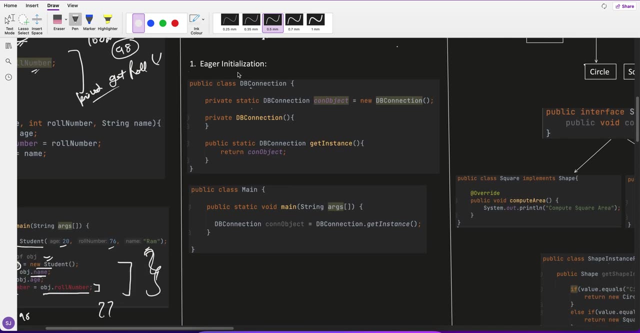 is, you can create only one object and then you can perform many, many operations out of it. so what are the different ways to achieve this? there are four ways to achieve this is eager, lazy, synchronized method and double locking. double locking is the one which is actually used in the industry. let's first see the eager initialization. so how you 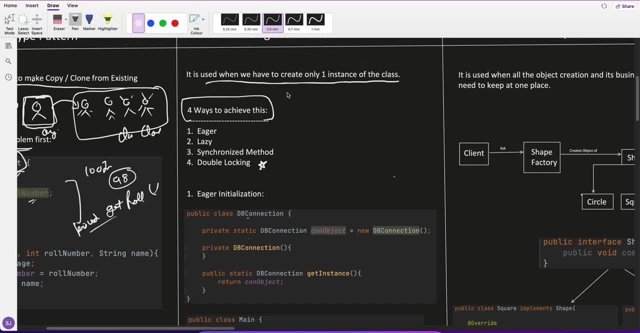 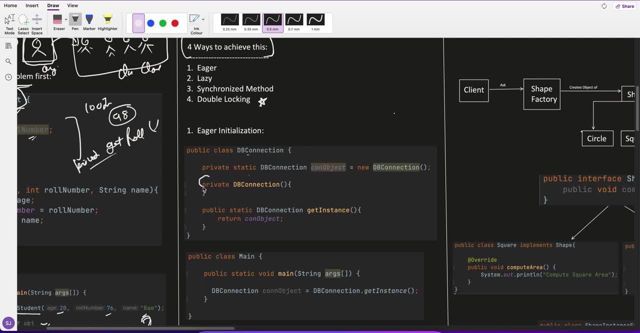 create a singleton pattern is: first you have to restrict the creation of an object. who is the responsible for creation of an object? constructor? so first you have to restrict it. how you can restrict it? creating the constructor private so that outside of this class no one should be able. 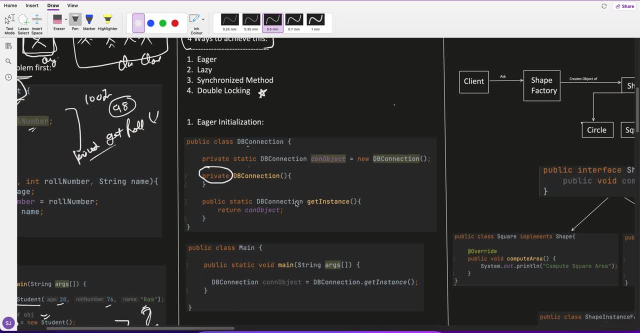 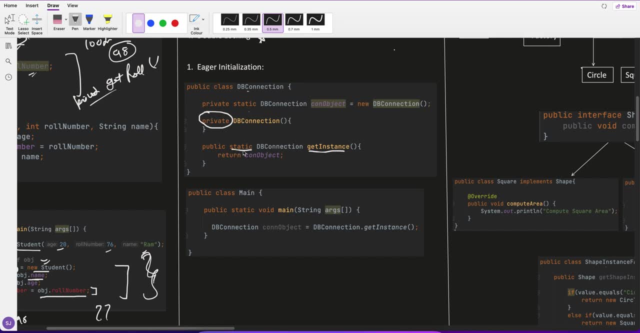 to call the constructor. okay, then you have to expose one method which other classes can call it. right, they can call it through class name. so that's why i made it static, so they can call this method and then this method will return. make sure that only one object is returned. so in the 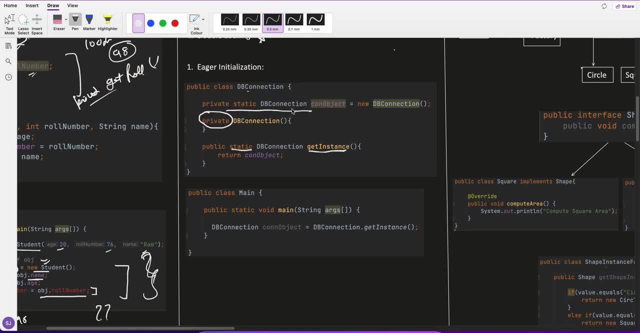 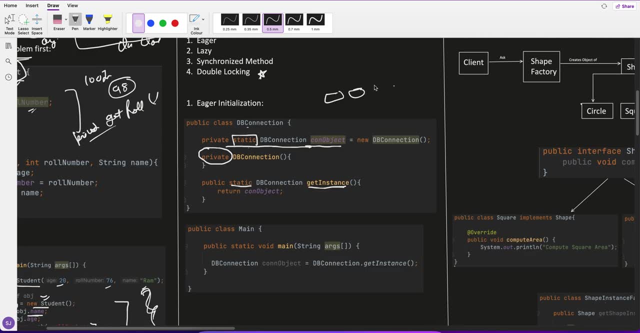 eager initialization in the instance variable. i create a static because this static objects are related to a class. let's say, even if you create so many objects, you know that static members are related to a class. even if you created 10 objects, this static variables are related to a class. it's. 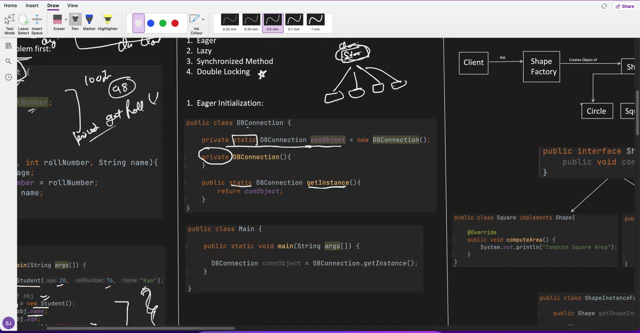 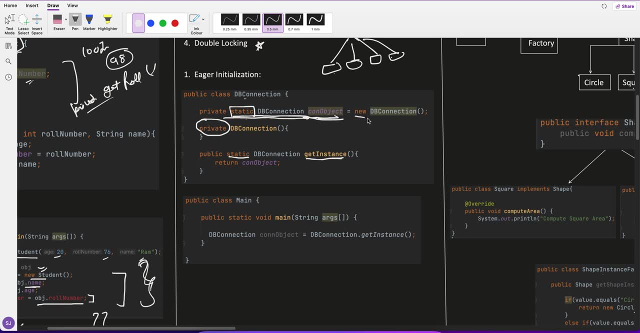 not related to objects. all 10 objects will share this. so first i have created a static object because now it is related to a class and i have eagerly initialized. it means when the class will load right, this static object will also get initialized. so at the time of loading itself, this variable is object one. 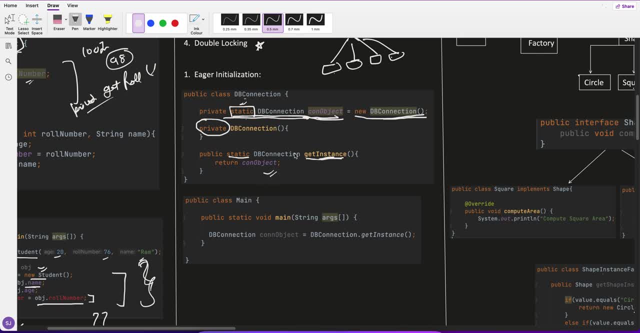 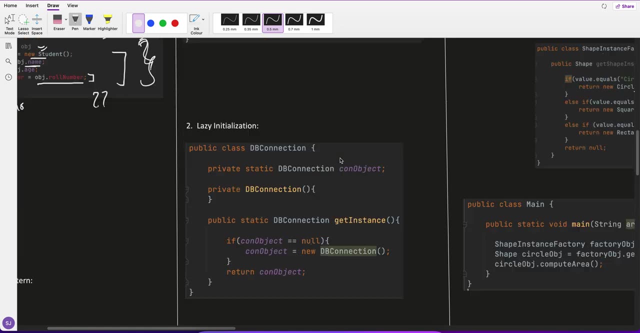 object is created. now in the get instance, i am just returning that object. it is not creating every time new db connection, new db connection, new db connection. it's just returning whatever we have created. that's why it is called eager. okay, so this is how you can call the get instance method. second is lazy initialization. in the lazy initialization 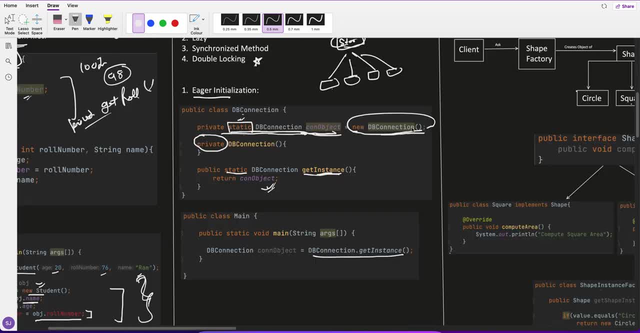 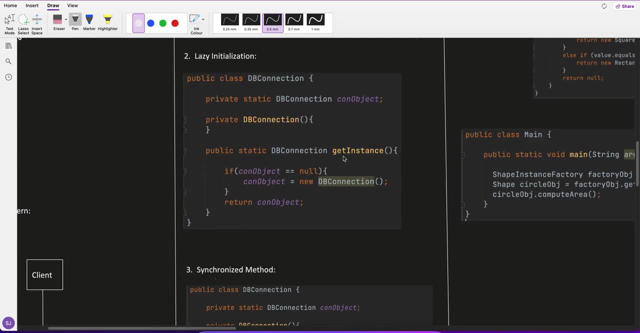 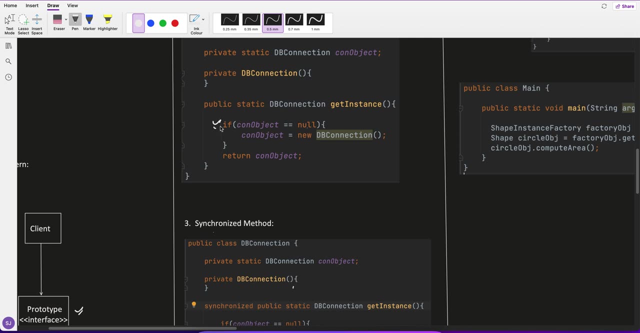 what we have done is, instead of at the load time itself, we want to create that. hey, whenever the method invokes, whenever the there is a requirement, then only create an object. so here we haven't initialized it, here we are initializing it in the get instance method. we are first checking it and 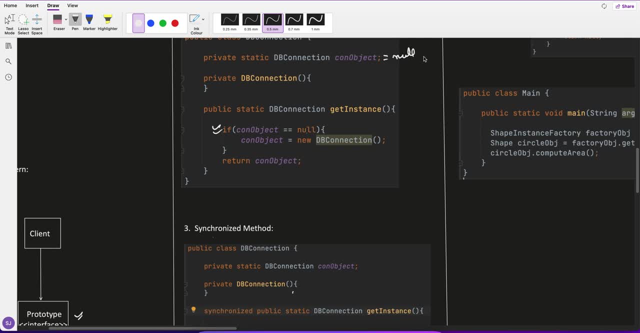 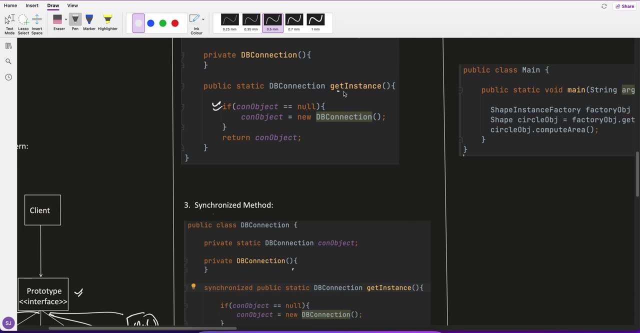 checking if object is null. by default it is initialized with the null value, right, because it is static. so during load time this will get initialized with the null. now somebody call this method, get instance, it will check: hey, object is null. yes, it will create a new connection. now it. 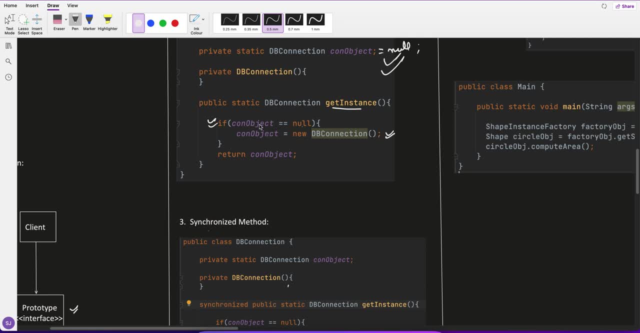 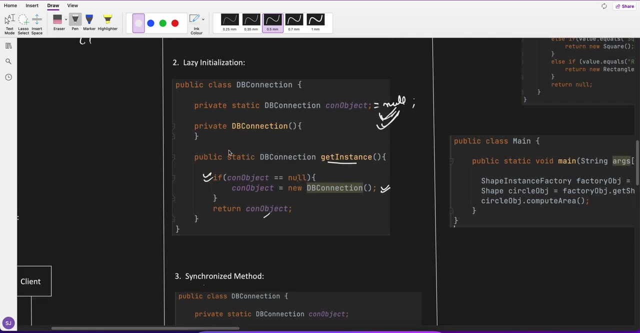 has a value. now the second one comes, it will say it is null, no value is already set. it will return it. but there is a problem with this in lazy, let's say, two threads directly comes simultaneously: thread one, thread two comes simultaneously. both will find a object. 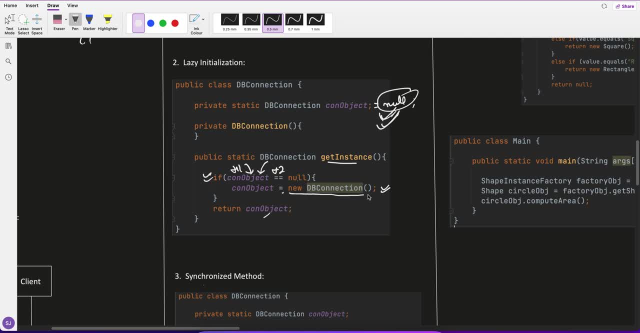 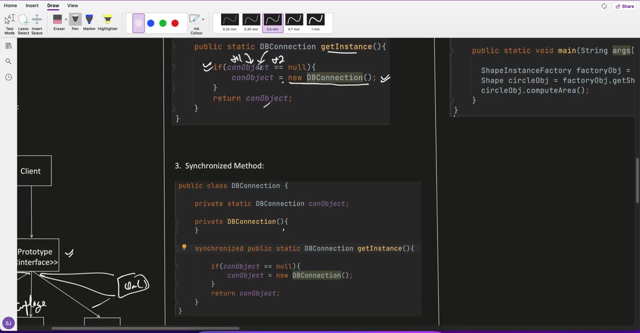 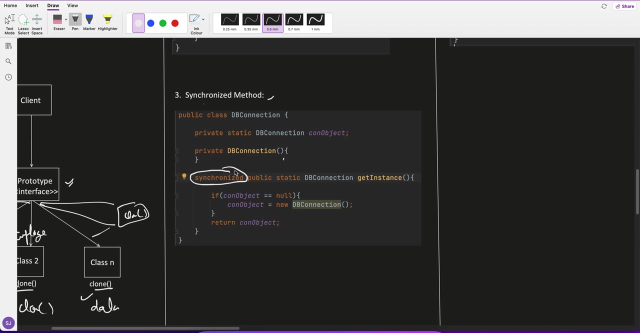 is null and both will go inside and both will call the new db connection. so two objects will be created in the memory. okay, so that is the problem with the lazy one and how it resolve it: through synchronize. so let's say i have put a synchronize over the method itself, so you know that synchronize. 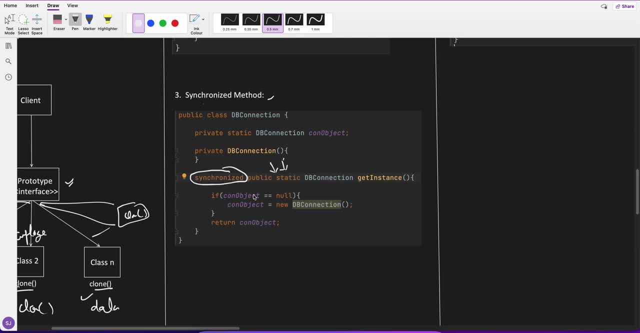 put a lock. so now two threads comes in, only one will go inside, so it is null. yes, for the first one it is null, it will create an object now. second one will go inside. hint, it is null. no object is already created. it will return it. but the problem with the synchronize. 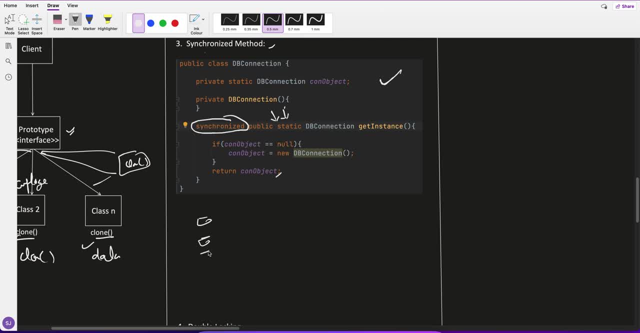 method. it is very expensive. let's say there are thousand requests coming for get instance. so first time it find it do a lock because method it's a lock on the method. it do a lock and then it is null. then it create an object. so it was, uh, null. so now it creates an object. now the second request comes, it again put lock, but the 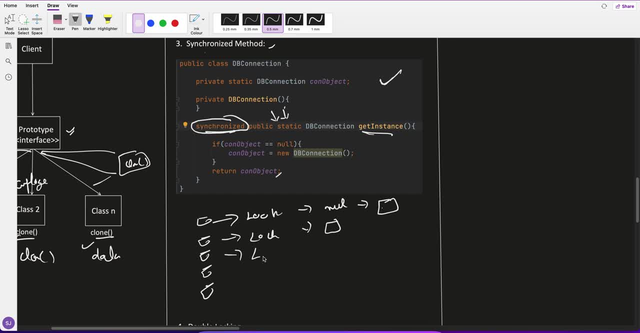 object is already created, it will return it. third, again put lock, because it's on method. since object is already created, it will have to just return it. but here, if you see that the locking is, you are putting, let's say, thousand, ten thousand times this method has been involved. you have to put lock every. 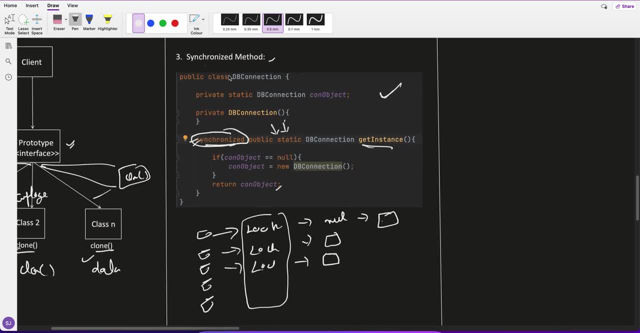 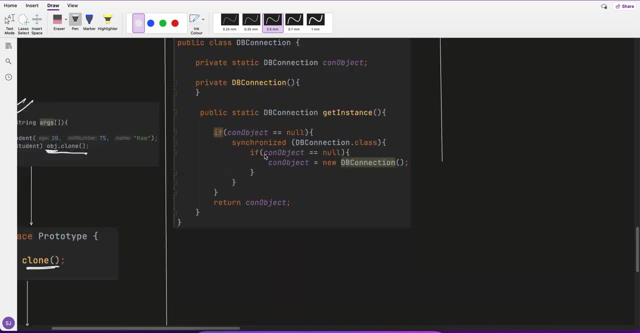 time and locking is very expensive method. so that's why synchronize method is never used. double locking is used. and how double locking has resolved the solution is so: first it put two times. check this. so how it put. let's say two threads comes in, t1 and t2. both comes simultaneously at. 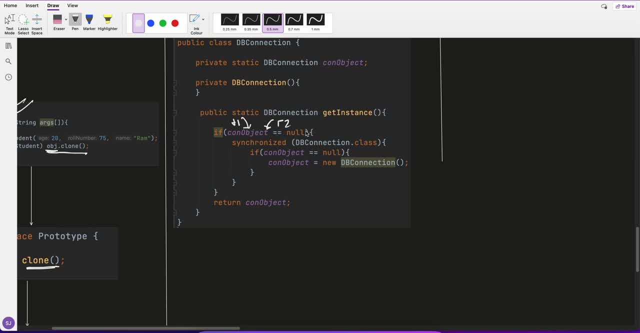 the same time to this line. if object connection equals to, equals to null, let's say it is currently null. yes, it is null, so now both will come at this step: t1, t2, that's synchronized. because of synchronize, only one will go inside. let's say t1 is going inside, now object is null. 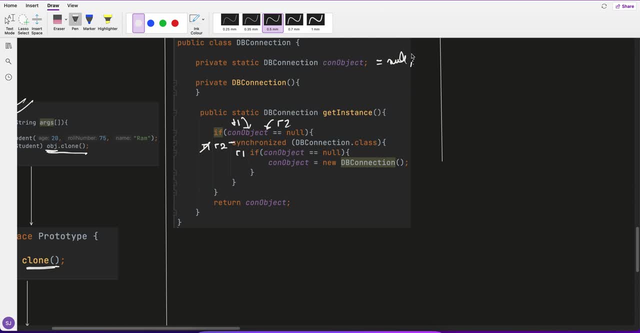 yes, it is still null. now it will create a new object. now the new object is created, okay, and it goes out and the lock is released. now t2 will take the lock and it comes here. now it is again checking. so double checking. is connection object equals to equals to null? no, connection object is already. 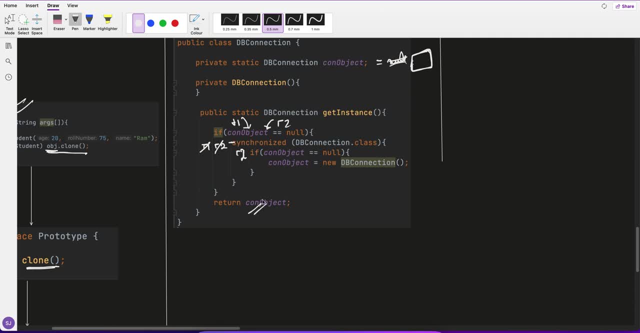 created. so it is not creating a new connection, it will simply return it. so here, if you see that we are checking two times, here first is here at the first time itself, before putting a lock, synchronize. we first check if there is already an object, return it. but because let's say simultaneously- 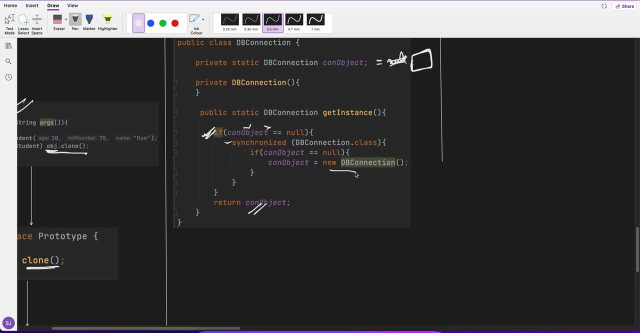 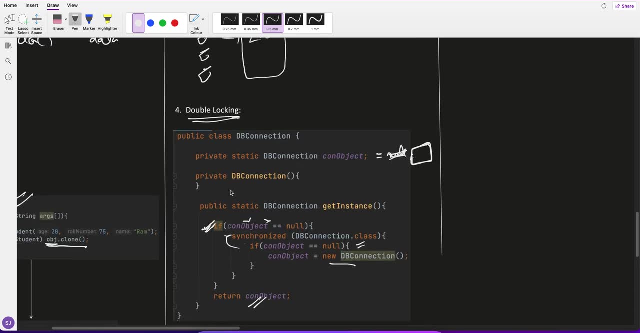 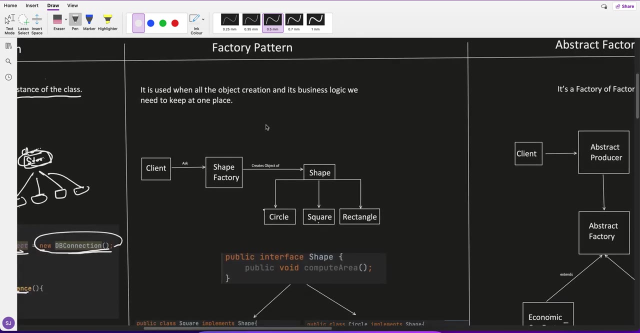 if threads comes and only one goes inside and created a connection and other goes, so there also we have put a check. if it null, then only created, otherwise not. so this is double locking and this is used in the industry. let's say factory pattern. this is very simple also why factory pattern is used when all the 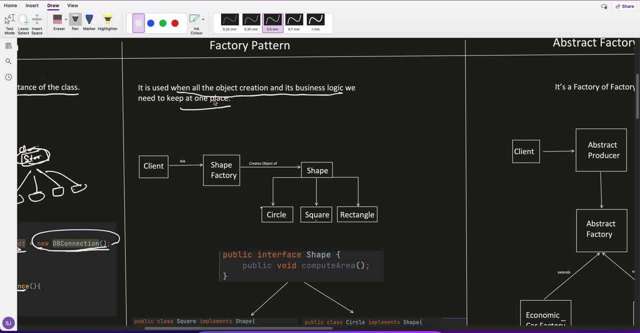 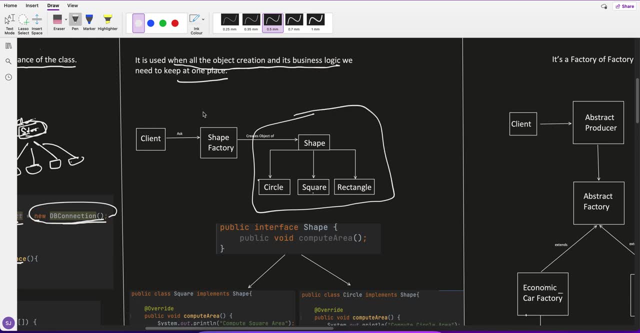 objects creation and its business logic. we need to keep at one place. consider this. let's say this is the object relationship you have in your class. there is no factory as of now. what problem it can come. so let's say there are thousands classes spread: class 1, class 2, class 3, class 1000. 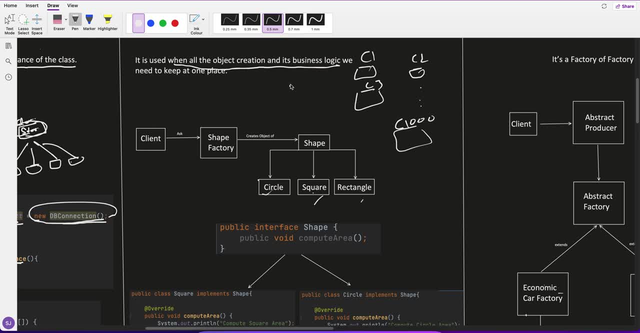 and are using this objects. let's say it is using new circle, new square. it is also using new circle, it is using new rectangle. First problem which can come in is like: let's say you want to change the logic of this creation of the circle. you want to have one condition. if certain condition is, 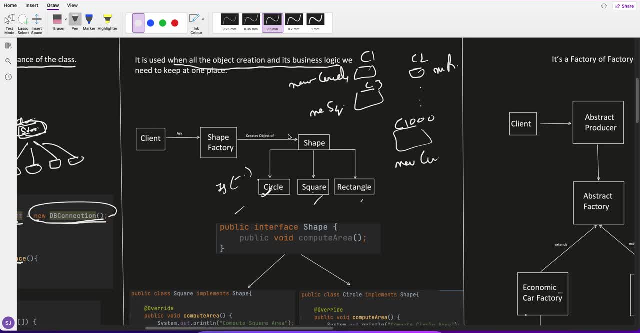 specified, then you have to call the circle. Now what I have to do is, on all the classes, all the places where the circle object is initialized, I have to put that condition: if certain condition initialize, then only created. if certain condition initialize, then only created. 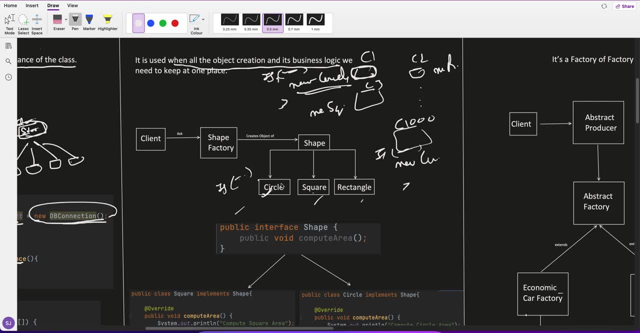 So you can only understand this from this example itself, that if the object creation logic is spread across the your component and if any change required in the logic of the creation, you have to change in all the places. So that's where fact factory pattern says that, hey, I will keep all the logic within my class. 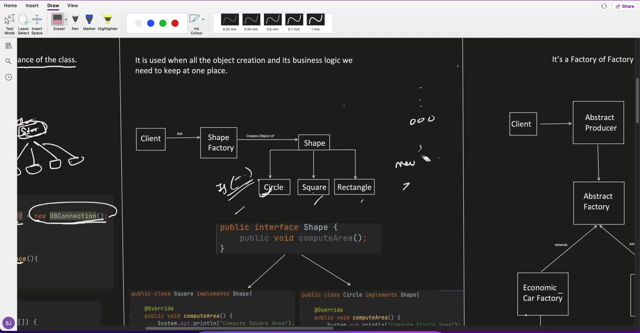 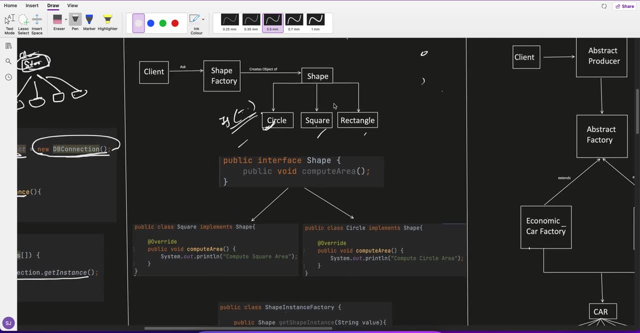 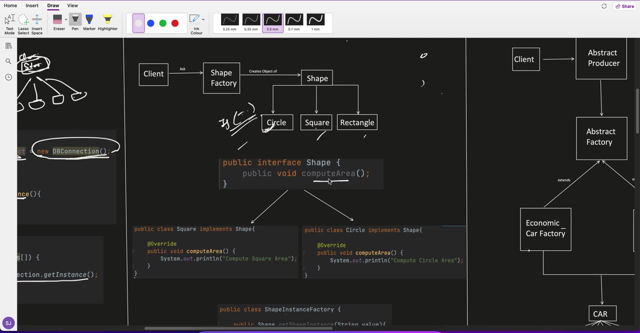 And if any change required, you have to change only at one place, not at 100 of places. Okay, how Let's see this? So I have created this structure, So I have a shape. shape has certain method. let's say, compute area. 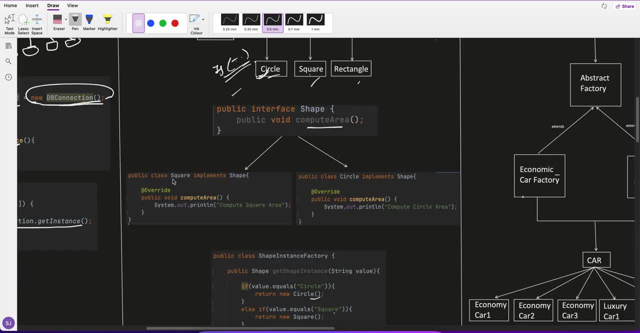 So now, let's say shape is as a circle, square, rectangle. So I have a square, it is computing the square area. I have circle, it is computing the circle area. you can have another which is computing the rectangle. here Now I have created a shape factory, Now I have created a shape instance. 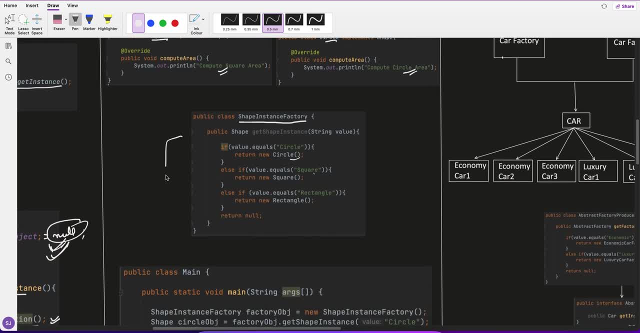 factory And it has one method, which is taking the responsibility of creating the object. So now in the input, based upon some input, okay, client want circle- object: I am creating a circle. client want a square: I am creating a square object. client want rectangle: I want. I will return a. 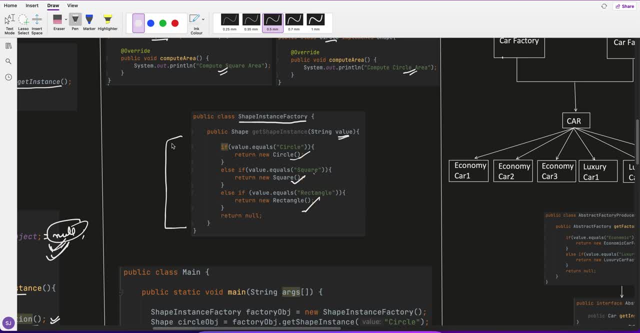 rectangle object. Now say, in future, any change in logic happen, hey, if well. so let's say: I want, I don't want another square object I can delete here. If value is equals to equals to rectangle, or value is equals to equals to square, I just return the rectangle. Okay, so now, if you see, 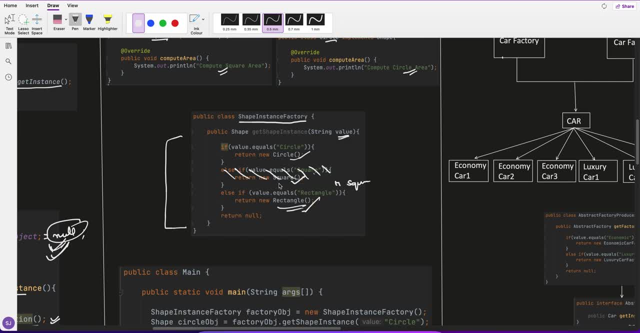 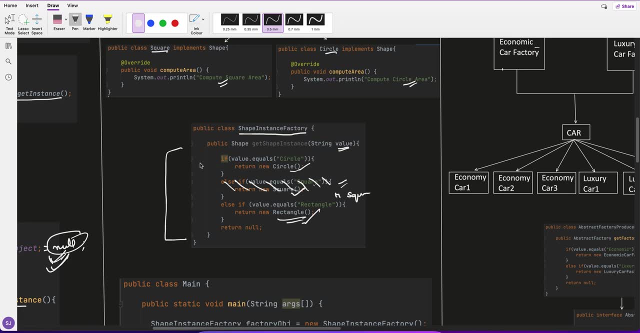 that I have to change only one class for the logic chain. I don't have to change the hundred and 1000 of classes where the square and rectangle are used now, Okay, so that's the benefit of getting a factory And how you can call it. you can create a factory object. 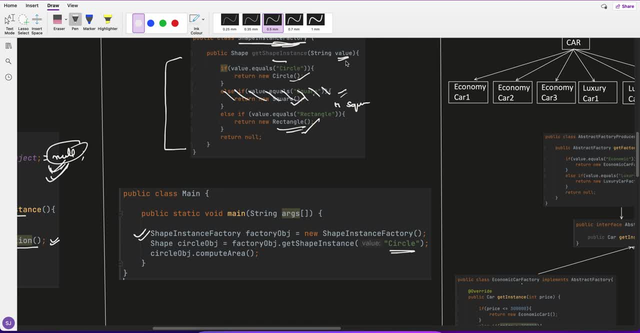 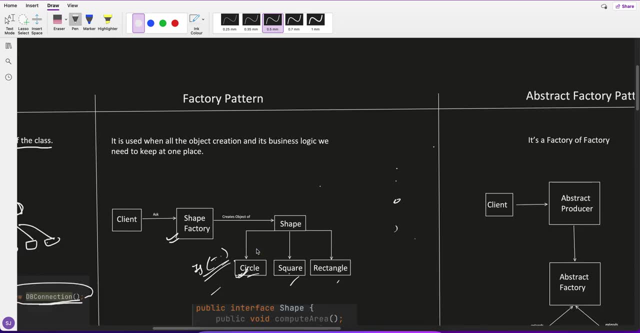 And then call this method And whatever the object you wanted, just pass certain value and you will get an object of it, And then you can compute the method. Okay, now let's come to abstract factory Pattern. abstract factory pattern is nothing but a factory of factory. 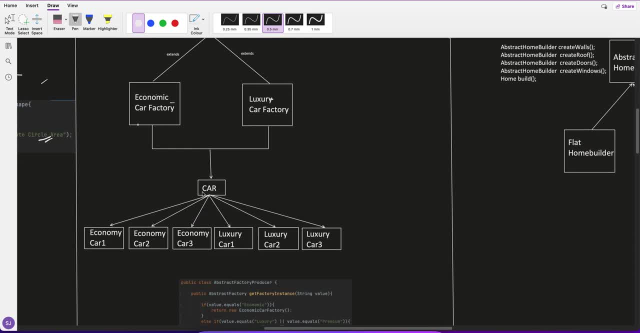 Okay, so now let's say i have taken this example car, so in the car, let's say car, i am manufacturing economic and also luxury. i have a different varieties of economic car: one economic car, two economic car, three. then different variety of luxury: luxury car: one luxury car, two luxury car, three. so instead of 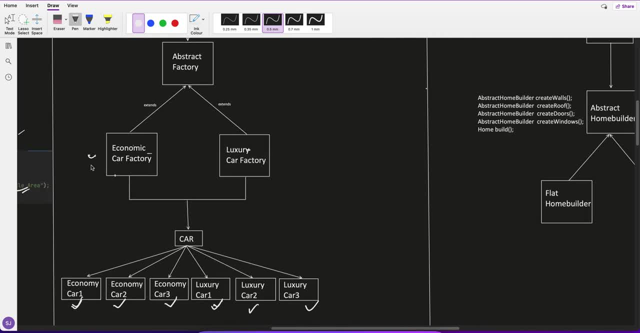 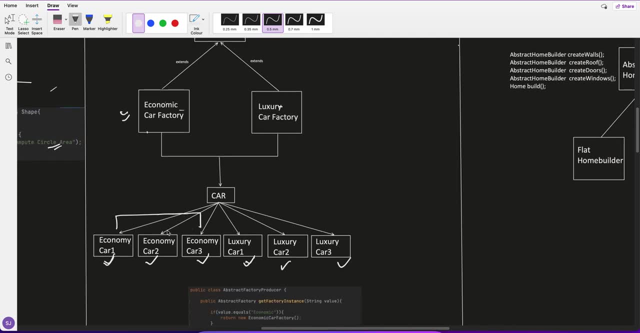 creating one factory out of it. let's say i have created couple of factors: economic car factory. so economic car factory, based upon certain logic, it will return objects of this economic cars only. similarly, luxury car factory, it will return the objects of this luxury car only right now. 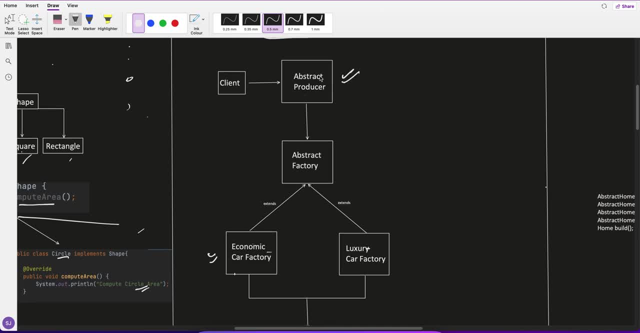 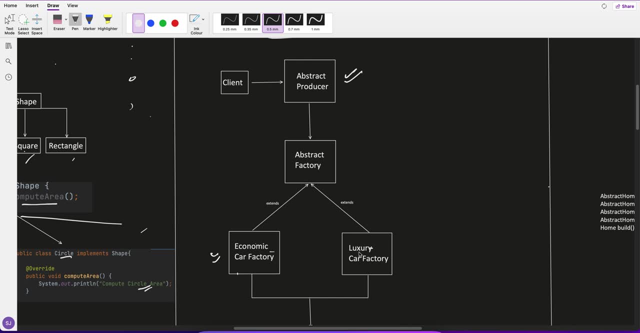 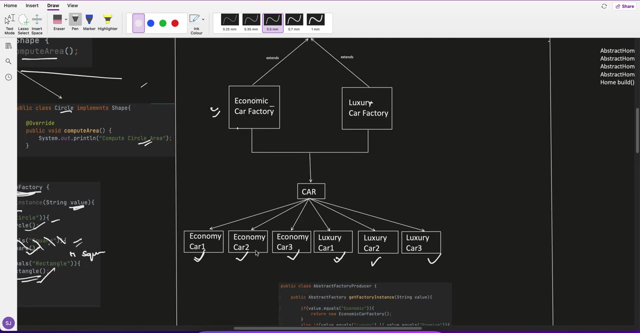 here i have a producer which is- you can say that- factory of factory. so here, whatever we are doing, it will first return which factory you wanted, either economic car factory or luxury car factory. okay, based upon that, it will return that object and from that you can get an actually car. let's understand with an example. 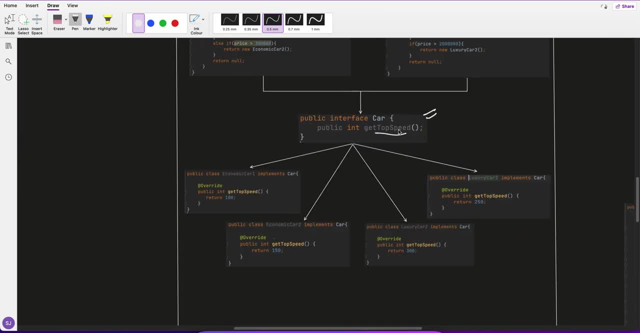 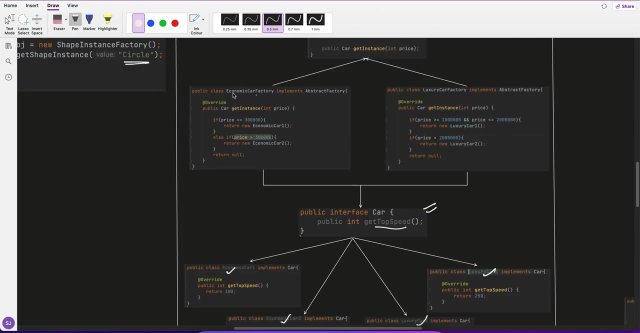 so this is my car and i have one method: top speed. i have created economic car, one economic car two, luxury car, one luxury car two. and they have their mention, the top speed, randomly, certain values. now i have created two factory out of it: economic car factory, which is a child. i. 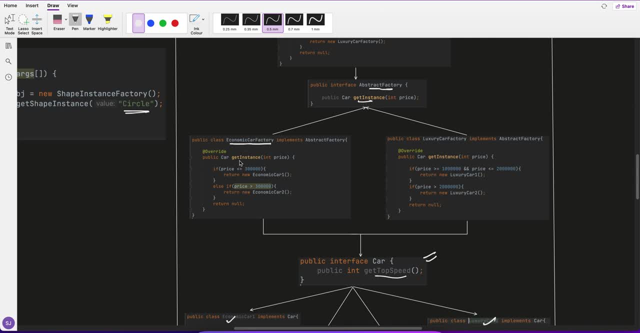 created a abstract factory interface so that this method can be same for both right. so i have created the abstract factory. get instance, right and the abstract factory. what it will do is get instance and based upon the price it is returning, economic r1 or economic card two. 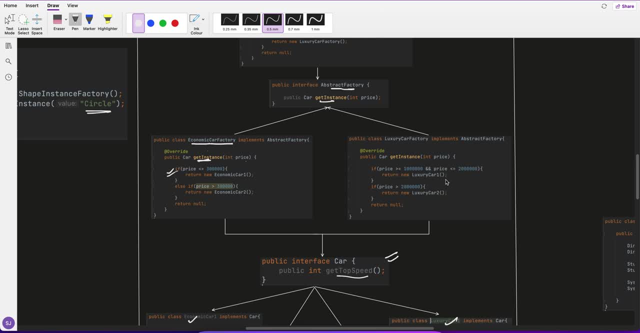 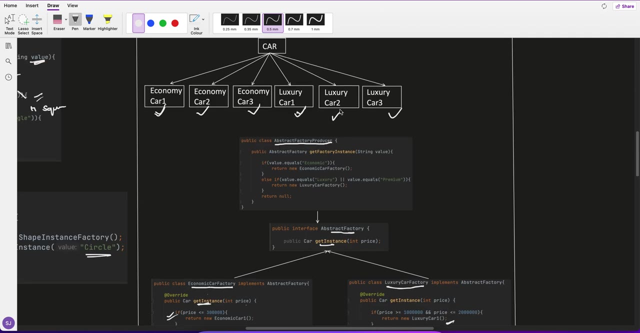 similarly, luxury car based upon the price, it is returning luxury car 1, luxury car 2.. so this factory is working on their respective cars, it is working on economic, it is working on luxury. now, if you see, i have created abstract factory producer, now based upon the value, instead of returning the original object, how it we were doing in the 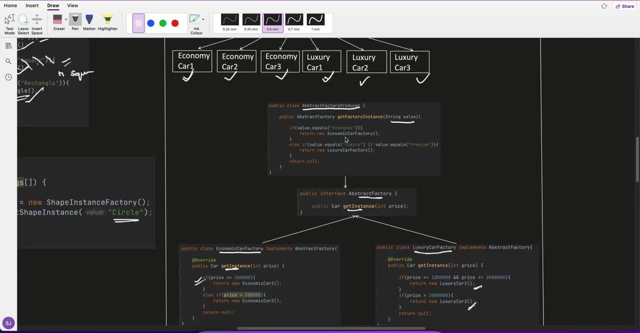 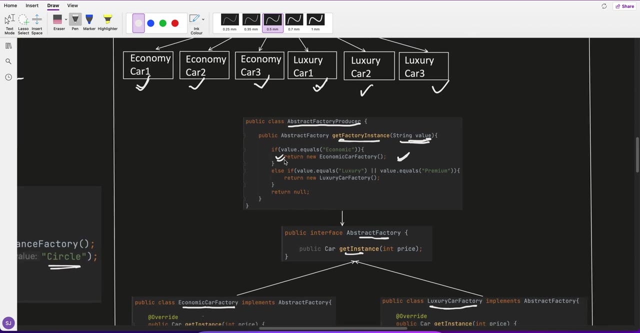 factory in the abstract factory, it will first return the another factory. so let's say, get factory instance based upon this. so let's say, if you want economic, if you want economic, then it is returning economic car factory. if you want luxury or premium or, let's say, valuable, 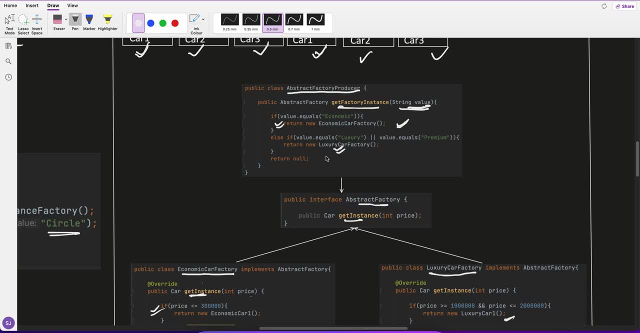 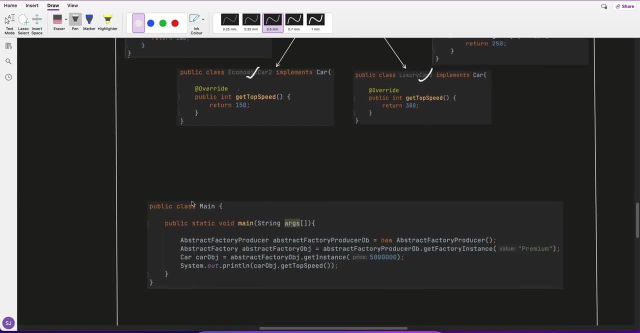 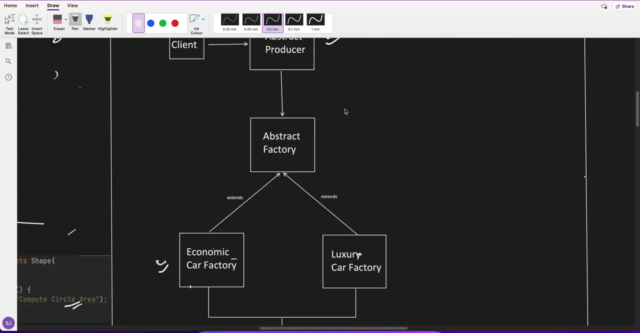 whatever the value would be. it is returning luxury car factory. okay, once you get the respective factory, you do your work. okay, now let's say how it we can work. so let's say: first, i am invoked. i created an object of a factory, abstract factory producer, this one, i created an object of this. so 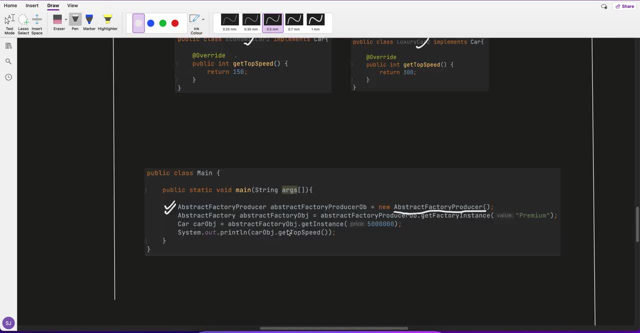 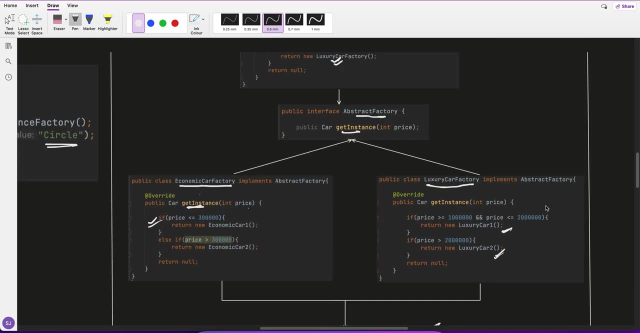 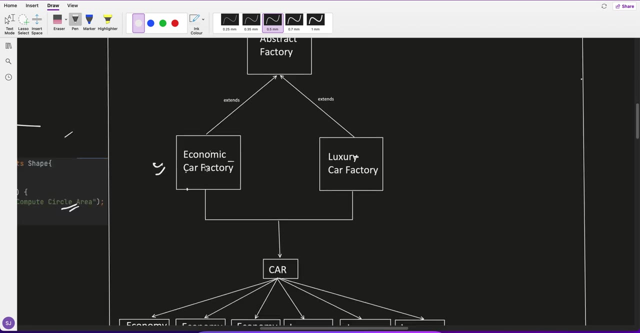 client created an object of this. then first i am doing is: hey, get, get me the factory of premium, so the premium factory is like it. what car producer will do based upon the logic: okay, you want premium, whether i have to return an economic car factory or luxury car factory, so premium. 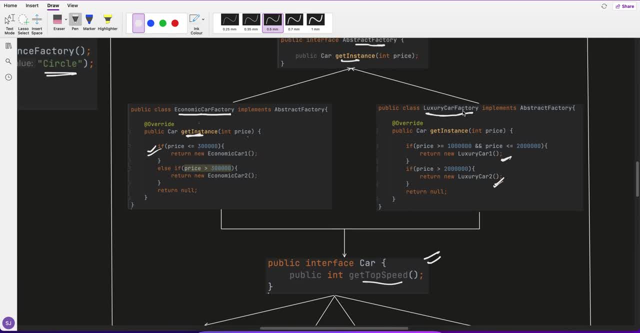 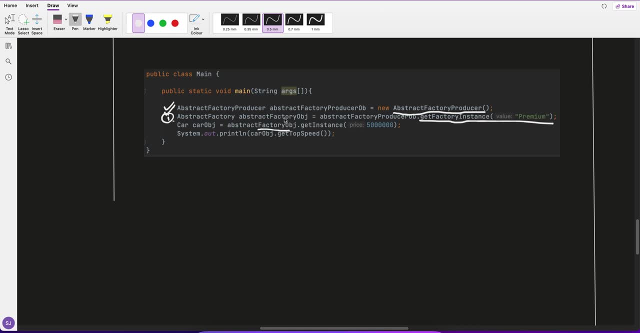 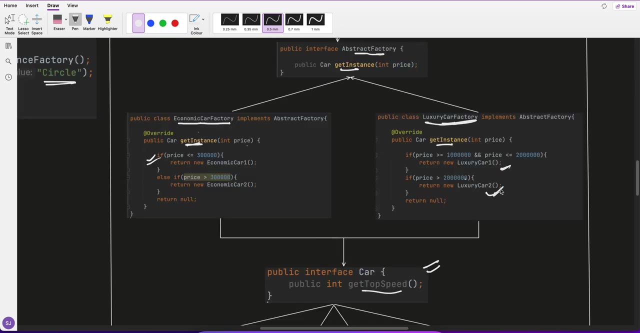 will return luxury car factory. so it will return the luxury car factory object. okay, luxury car factory object it got then from the luxury car factory object, whatever it returned, i call the get instance. so it will call the get instance method of this one and, based upon the price, it will return the actual car. 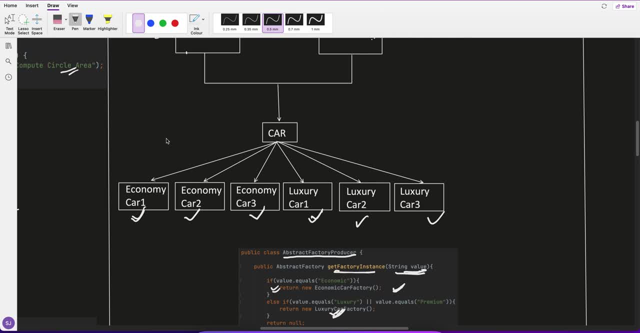 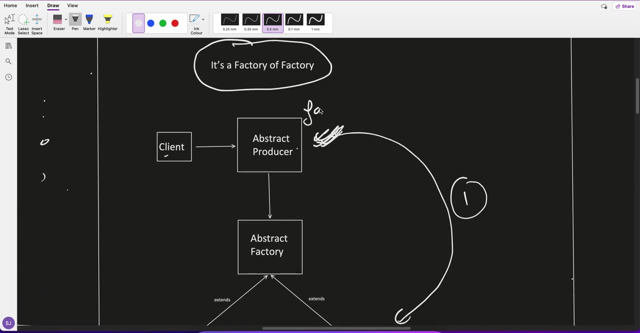 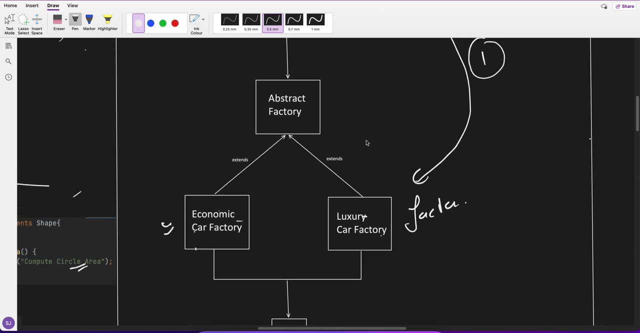 it returned the actual car. okay, that's why it is called factory of factory. so first it will return one factory. this is the first step. so this is itself a factory. this returns a factory, and this itself is a factory. okay, so it's a factory of factory. that's why it is called, let's say, builder. 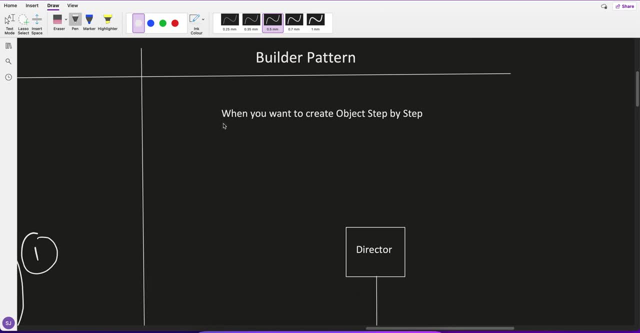 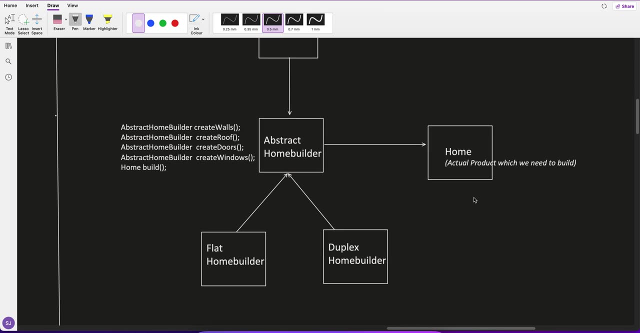 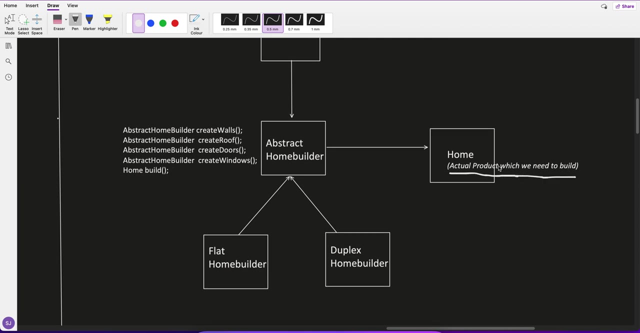 pattern. so builder pattern is also easy. when you say that, when you want to use it, when you want to add it or go from a designer to a designer type of build, what we are going to do is: you can geen demo bein 개 is, is, is. 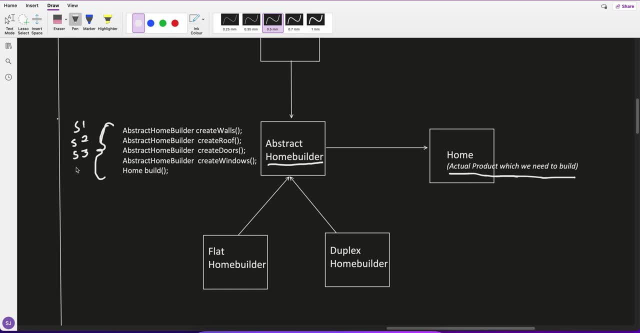 is is is: third step is create door, fourth step is create window and after this, all the step, ultimately the home is done. so this is your home builder. so, but let's say your home can be of different type: flat, duplex, villa, different types. so certain steps, implementation could be different from. 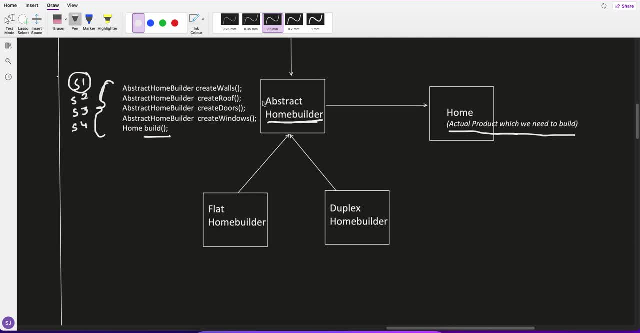 different types of this thing. so that's why you can have it as an abstract home builder. and let's say these are common for all the childs. so you can have defined this implementation of step 2, step 3, step 4 here: create roof, create door, create window, but create wall. let's say: 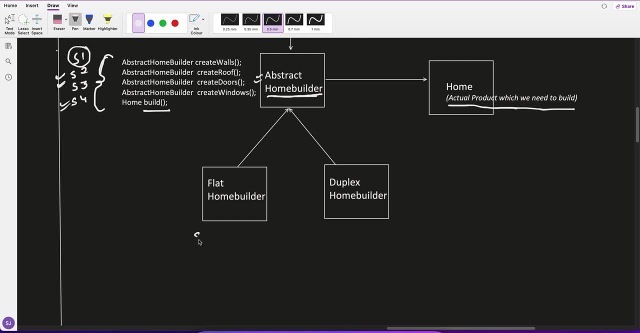 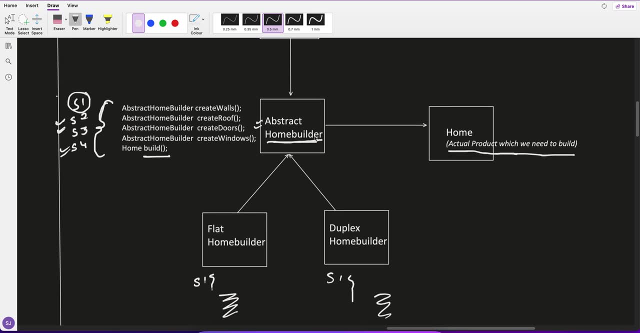 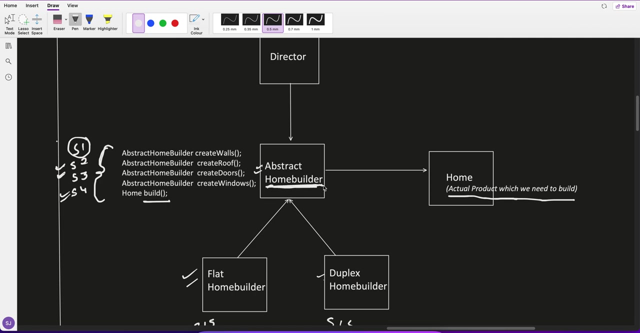 it is different. so each type of builder- flat builder- can write its own logic for step 1 right. so that's why we, generally home builder, keep it as an abstract so that in future any type of home builder or any type of value comes, you can extend it and override the behavior. okay, but generally the home builder purpose is: 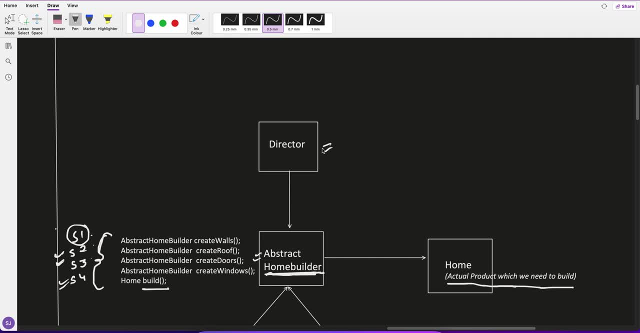 to implement the steps and director step is to orchestrate that. maybe for some use case, step 1 after step 2, step 3 has to be done. maybe for some use case, step 2, step 4, step 3 and then step 1 has. 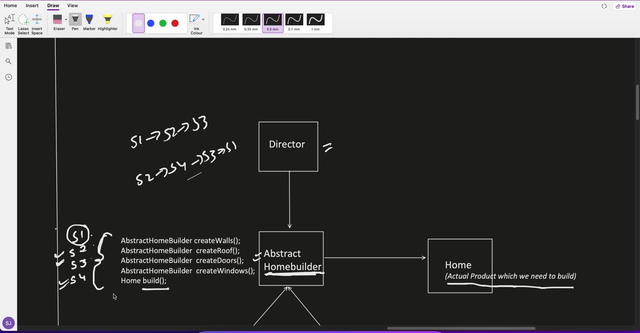 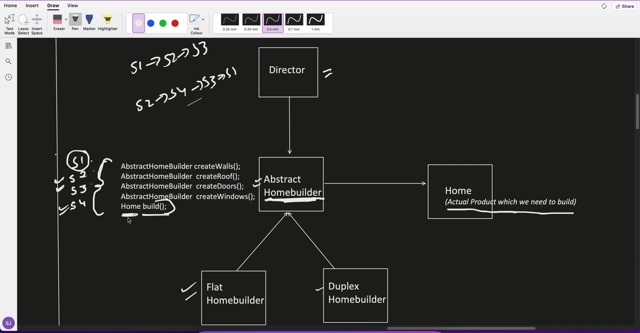 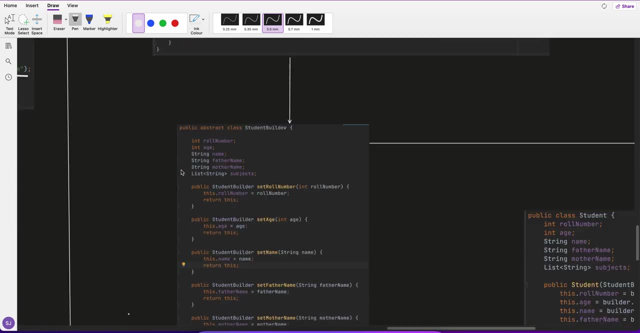 to be done. so, director, orchestrate the steps and the steps logics are present- into the builder and after all the steps done, there is a build method with actually return the product. okay, let's see understand with an example. so this is my ultimate student of a product which i want to. 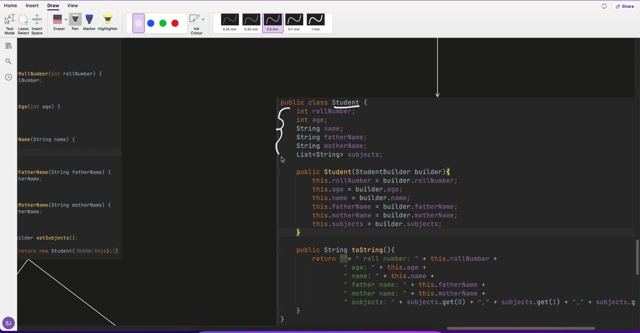 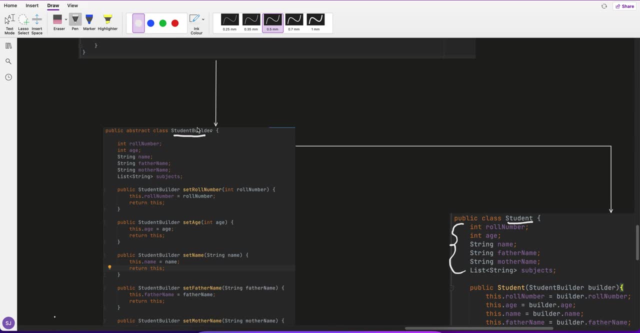 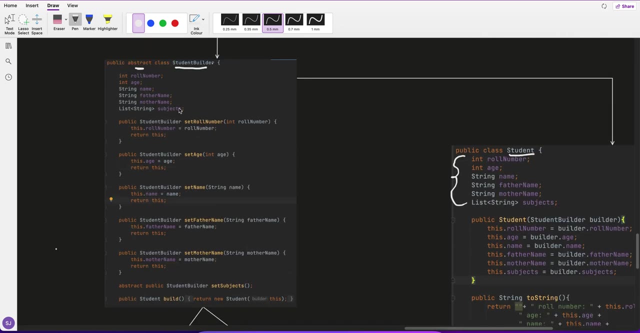 create. okay. so let's say it has certain parameters. i want to create in steps. so i have created one builder, the student builder. i have created an abstract because students can be able to create an abstract. other Steps: you have different type engineering, mba. that's why. so there are certain. 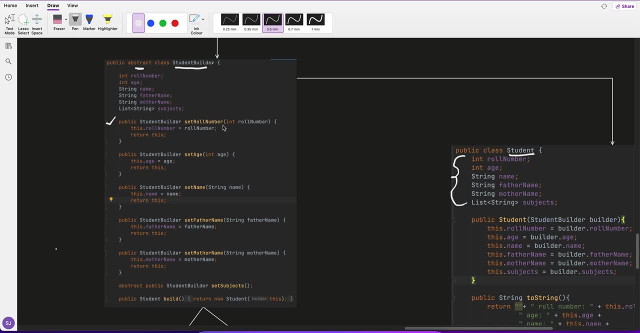 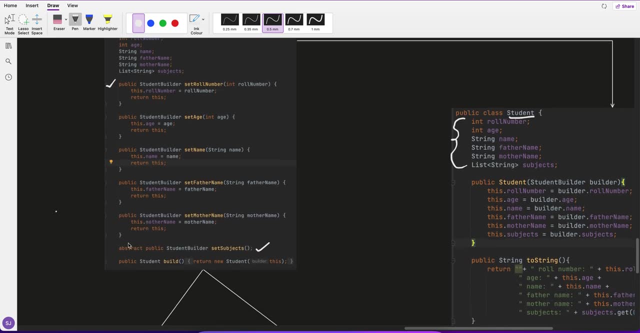 steps to create it. let's say I have step before. if you want to create a student, one of the step is: set your roll number, set the set name, set father names, set my the name, set the subjects. so if you see, the subject for each type of student is different. so that's why I make it abstract. 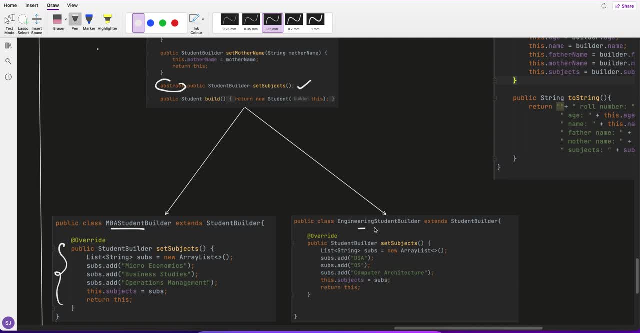 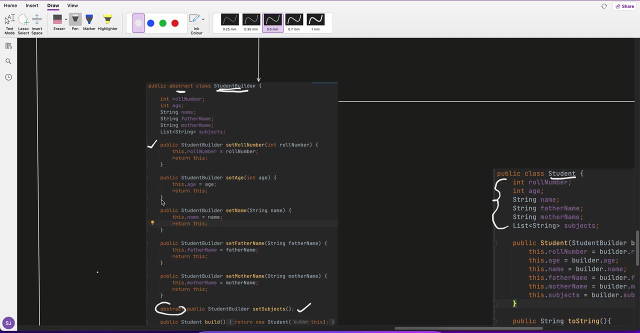 that okay. MBA student builder will override its own set subject. engineering will override its own. okay, but now what the purpose of builder? build 연습 is most important. we just have to seguir doing this and students can- will overwrite it. the purpose of builder is it has the implementation of all the steps. Okay, but here one thing. 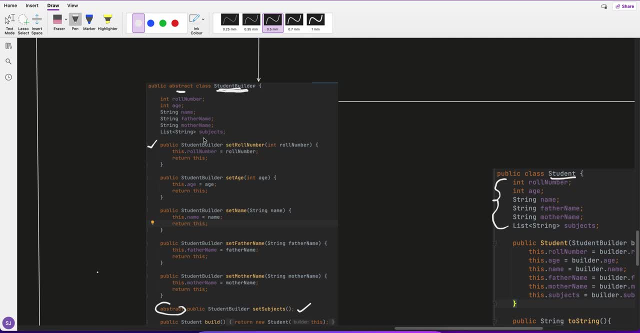 you have to understand is in the builder, till all the steps. everything is in mediator, not completed phase. So set roll number. it will set the roll number in the builder. Builder has exactly the same property as a student- the ultimate product- So it will set the roll. 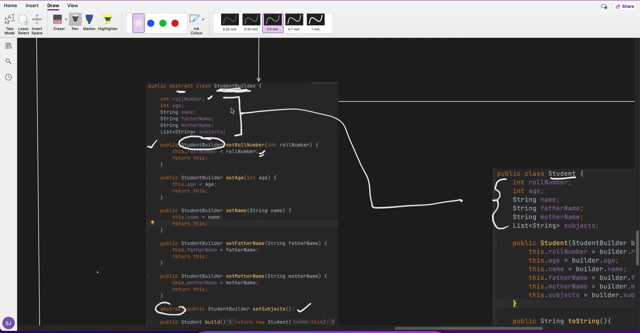 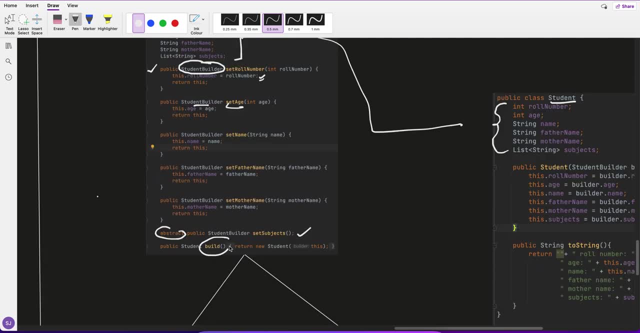 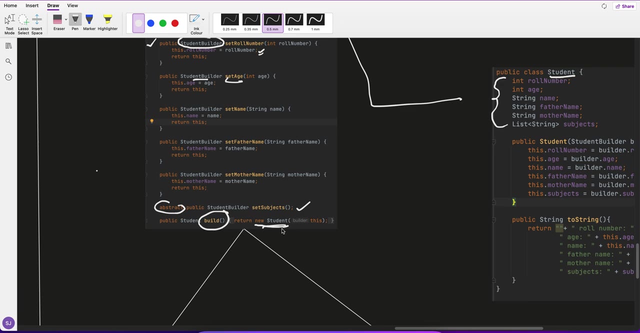 number, but what? it is returning again the mediator from builder. it will set the age, but it will set the builder only Ultimately. when, ultimately, the build method will be invoked from this builder, it will create a final product Right. So now let's see with an example. 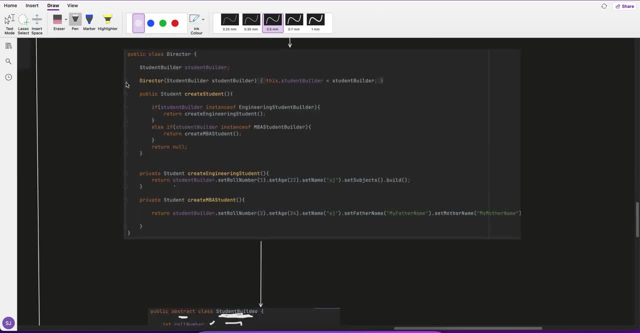 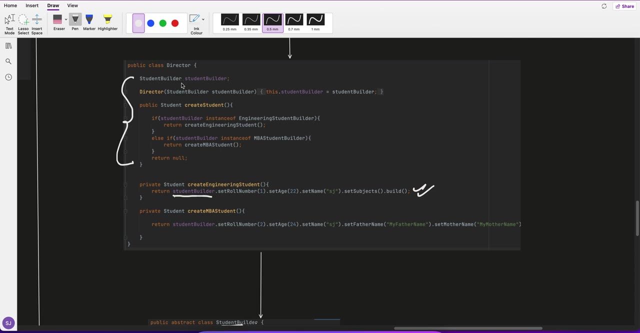 of here how it is called and director is: see director. I have created this just for understanding this method, But ultimate purpose of this is this: Let's say you want to create an engineer, a student, So you have a engineering, a student builder. I have used a dependency inversion So that director can have either engineering. 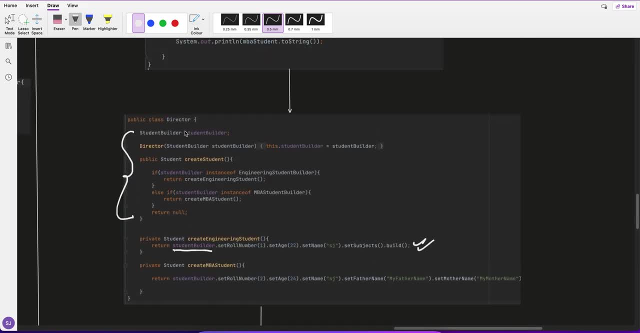 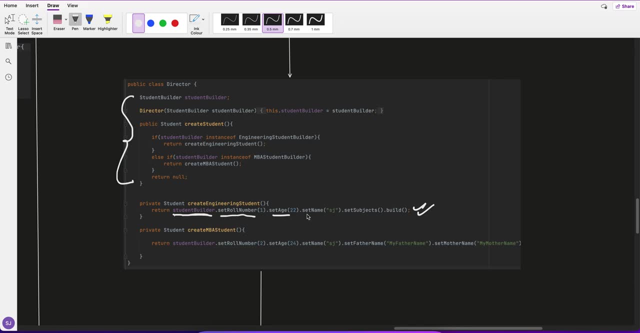 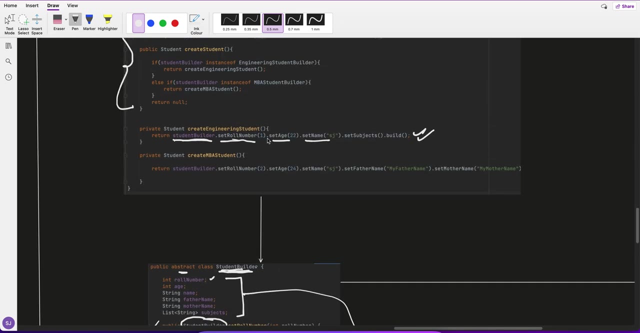 a student builder or MBA student builder, anyone right, based upon whatever the client wanted. First I set the roll number, then I set the age, then I set the name, So see set roll number. So set roll number what it written. again the string builder, then a string builder. 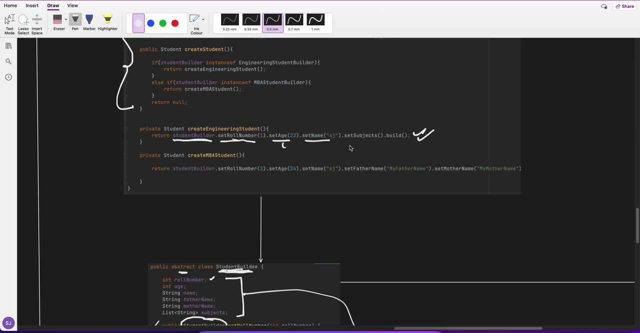 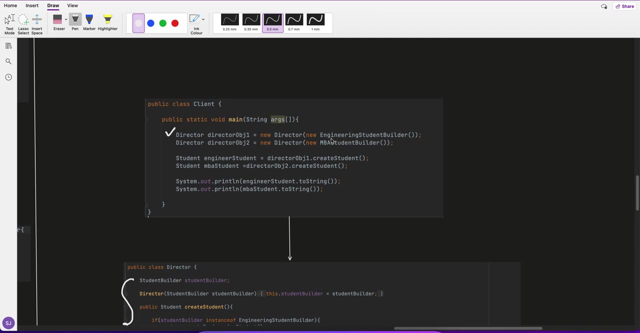 and set age. So here currently it's all in mediator phase. After everything is set then I call the build method Okay, then ultimately it returns the student. So let's see this. So first I created a director object for engineering, a student builder. I created another object. 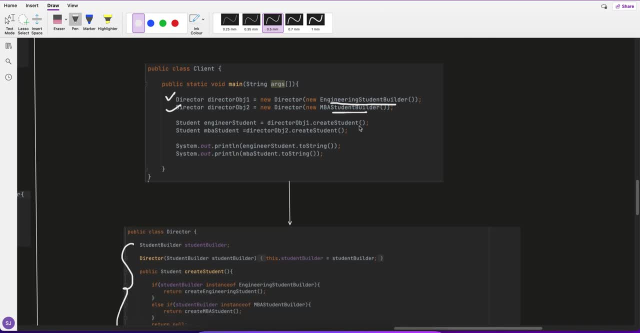 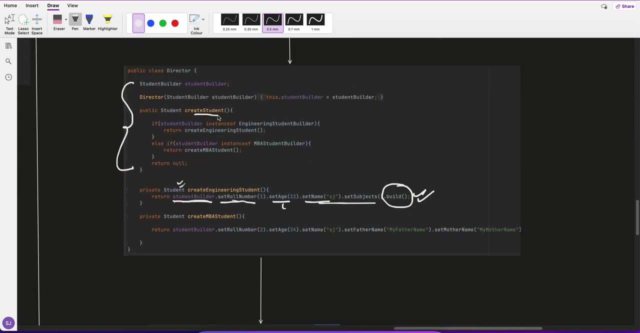 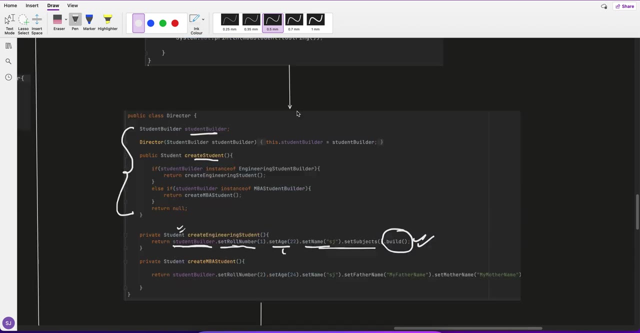 with MBA student builder, Okay. And then I call: okay, object one: dot create a student, let's create a engineering, a student builder. So it got a create a student and it say that, okay, this builder is engineering or MBA. object one is your engineering, So it calls the engineering one create engineering a student, So engineering. 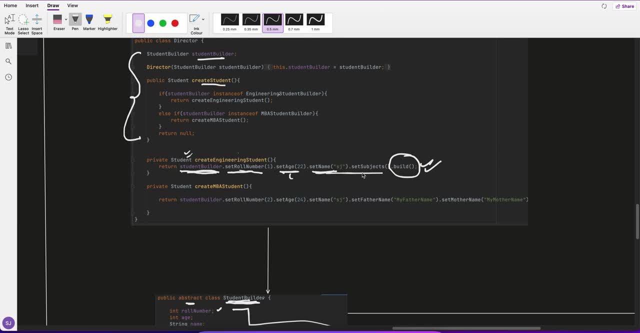 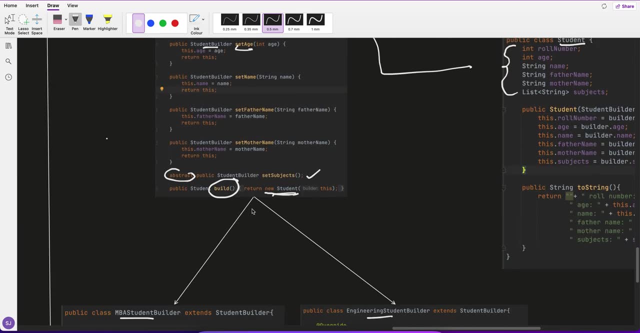 a student builder Now. it will set roll number, set age, set name, set subject. So till till. it is here, it is in a mediator form And ultimately, I set the build. And when you set the build, it will create a new student and pass this builder to an ultimate object. 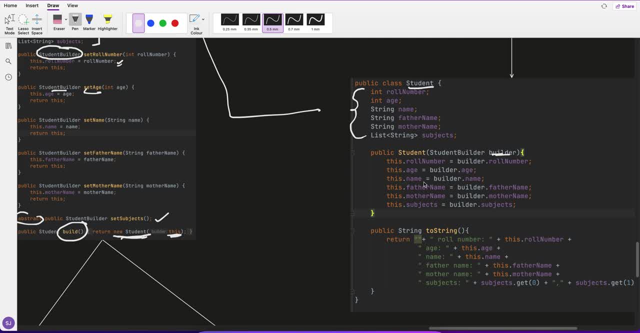 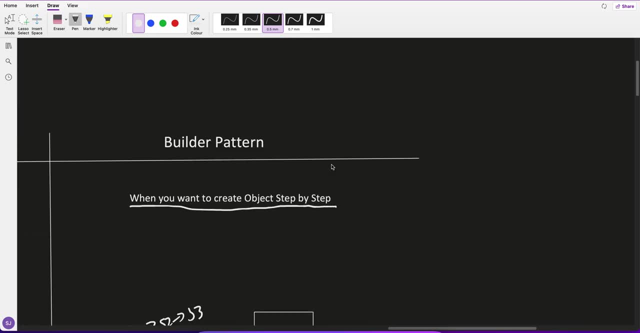 And from there it will create a original student and return it. So the complete in depth of builder. I have already explained dedicated video. This is I want to give you a quick remind and overview. What was builder pattern? a step by step creation of an object. 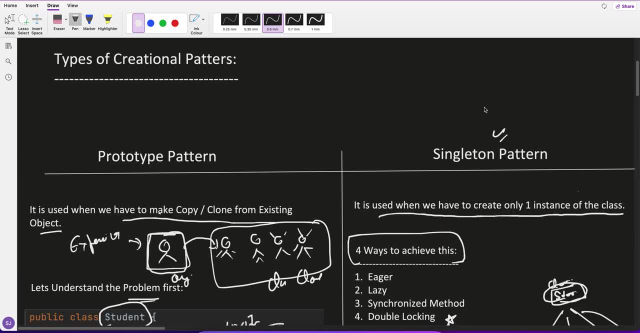 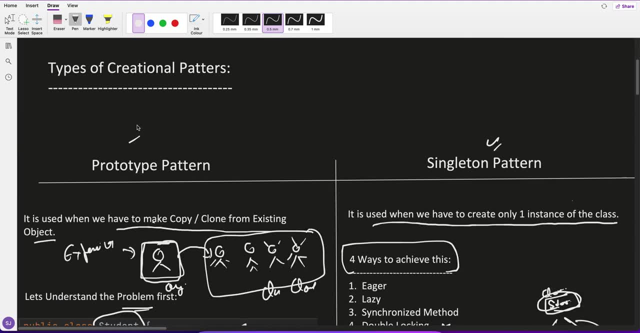 But yes, for each of this one you can check out the dedicated video And if, in prototype, you have any doubts, like it's a very simple and please feel free to ping me also. And this is UML coding and all. I have given the description and given this in the description. 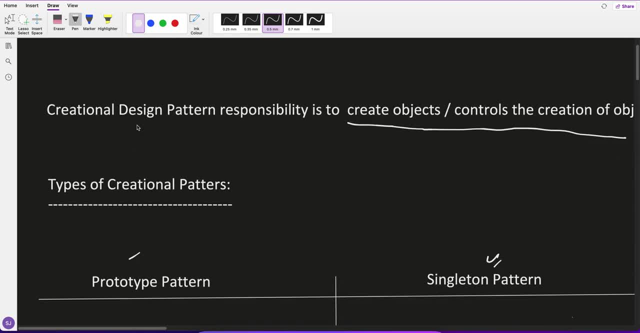 section you can check out. you can download it if you require. Okay, guys, if there is any doubt, let me know. Have a good day, Bye. 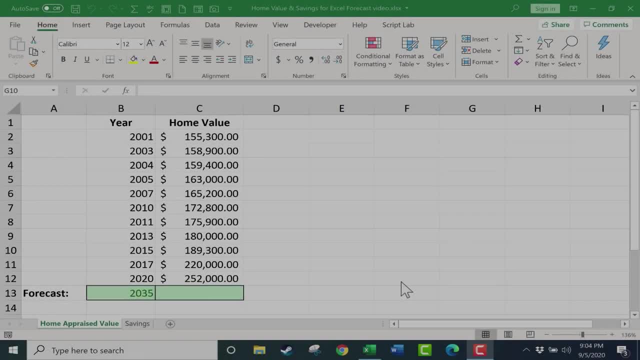 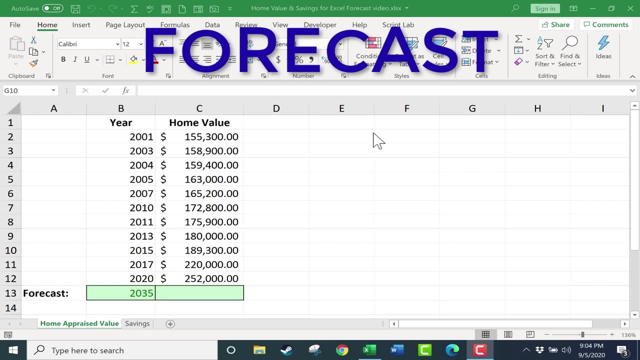 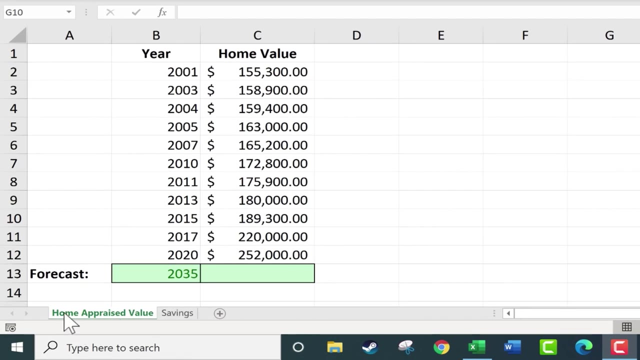 In this tutorial I will show you how to use the Excel forecast function, And this is just one way you can use it, but I think it'll help you get a sense of what it's for. You can see the workbook that I have here. It consists of two spreadsheets, one on a home. 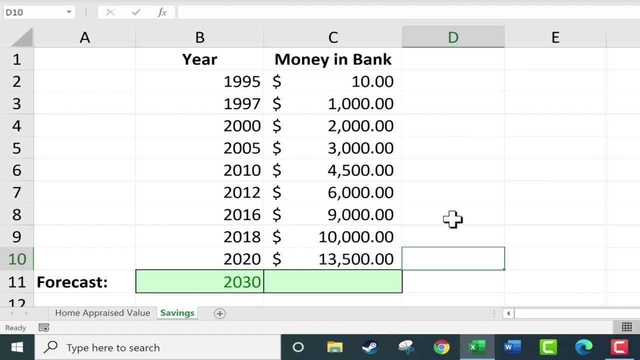 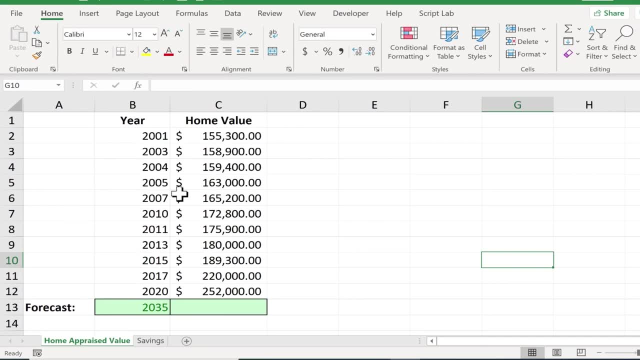 appraised value and the other is savings. It's like the savings account in a bank. Those will be our two examples. So here on the home appraised value spreadsheet, you can see I have a list of years. Let's say I bought a house in 2001, and this is what it was worth. 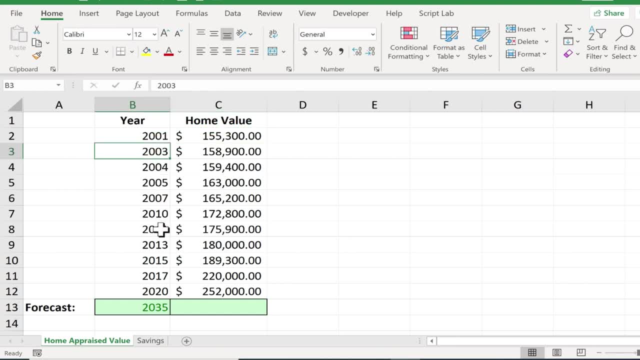 at the time And then maybe every year or two or three, the house got appraised. But each of these years has a different home value for the home. And these years are all in the past, of course. But what about the future? Is there a way to kind of forecast what the